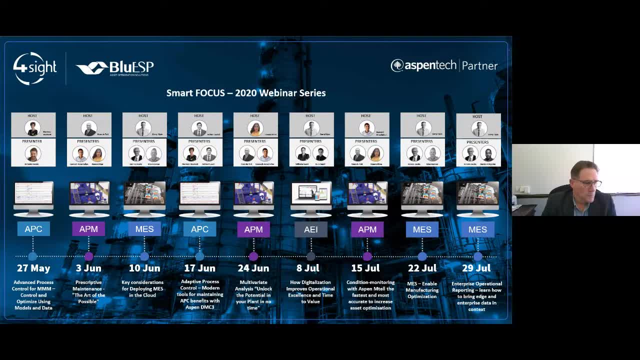 Hi there, Good afternoon, everybody Very excited. Wilhelm Swart here from Blue Espy in South Africa, sunny South Africa. Yeah, like everybody else in the world, we're also in lockdown, you know. so, being at five now, we're in four. From 1st of June we'll be 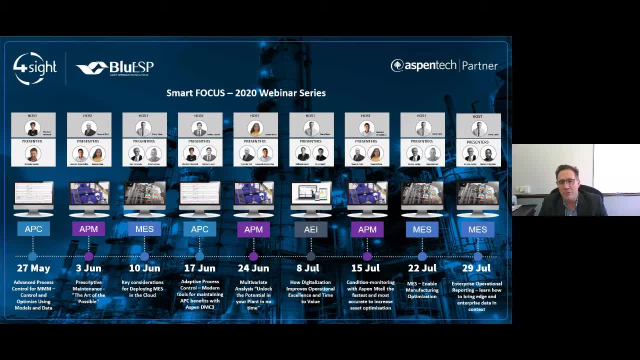 in lockdown three. So yeah, but we also just thought that we'll make this lockdown period very, very, very efficient, very productive, And thus we launched this webinar series, this nine-week webinar series. So the key focus is before and during the lockdown you. 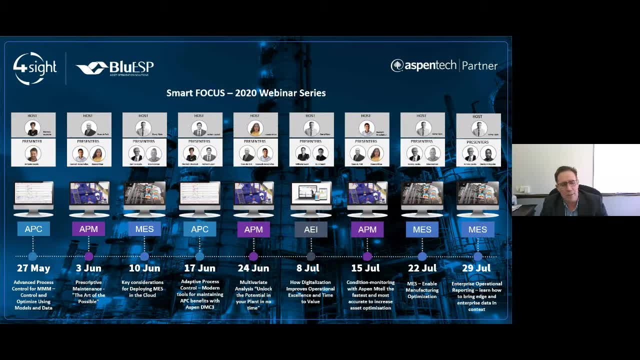 know there was a lot of. you know and even after there's already quite a big move to more remote operations. you know less eyes, less ears on site. You know the environment is very volatile and uncertain and ambiguous at times. Clients are looking for more agility. 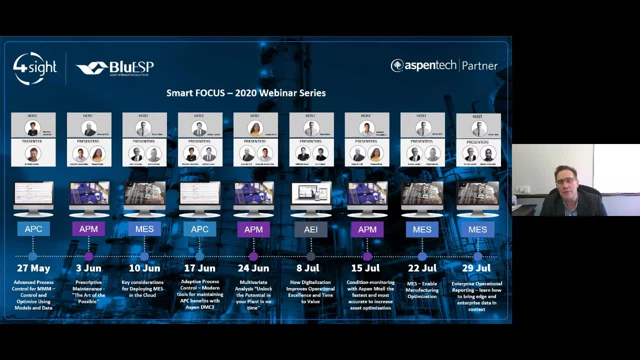 in their projects. There are fast turnarounds or paybacks like three to six months paybacks in a digital transformation project, or really. you know otherwise, don't do it. You know more focus on data analysis, more cloud, more embedded AI is the norm of the day right now. Much. 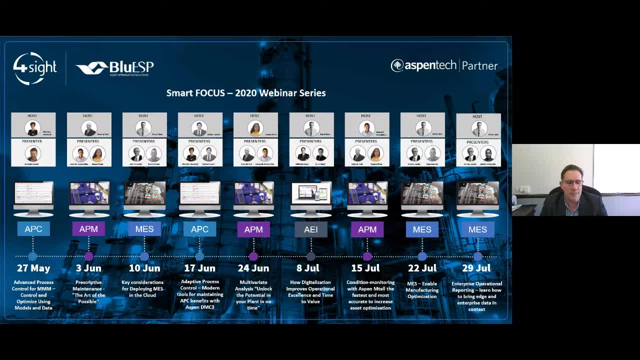 more collaboration between various vendors, various business partners, also with the end users and with the various parties at stake. So, yeah, I think it's a very important time to all you know, prepare ourselves. So you know, we at BlueSP- but we also use this webinar- 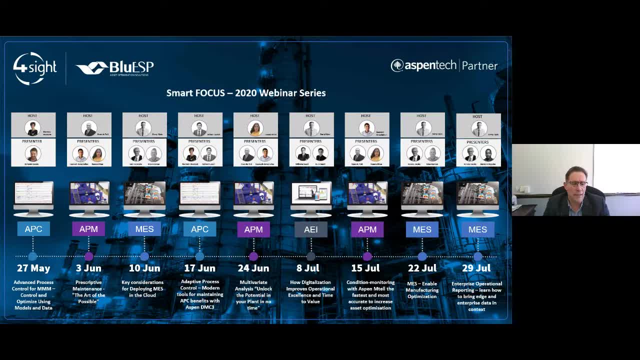 series to help our clients to upskill and cross-skill and to learn about, you know, using these intelligent agile technologies that we are going to talk about today and that we bring to you in this webinar series. So there's a continuous focus as the Aspen. 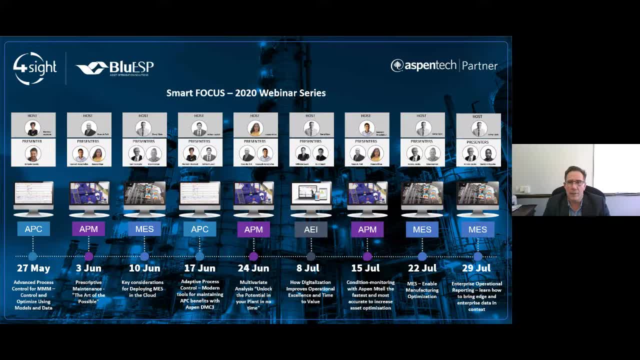 Tech CEO talks about. you know that we need to run operational assets safer, greener, faster and longer in this period, And that's what we focus on. So, as you can see on the screen here, you know we're bringing in three key themes. 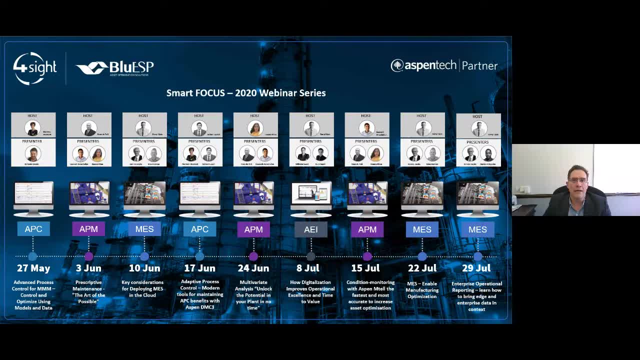 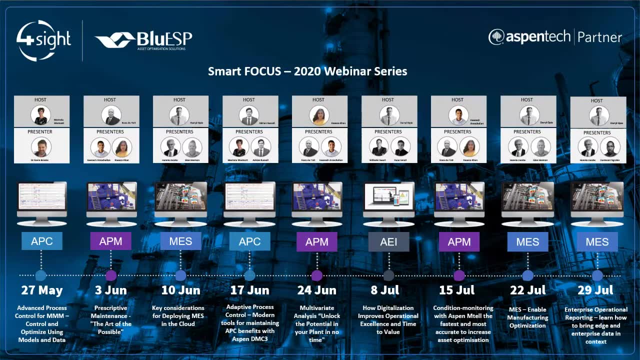 to you. So basically, firstly, you know the APC team, the Advanced Process Control team, will basically start today. They will. you know this team has just finished commissioning large projects in Canada. busy with projects, migrations in South Africa, various benefit. 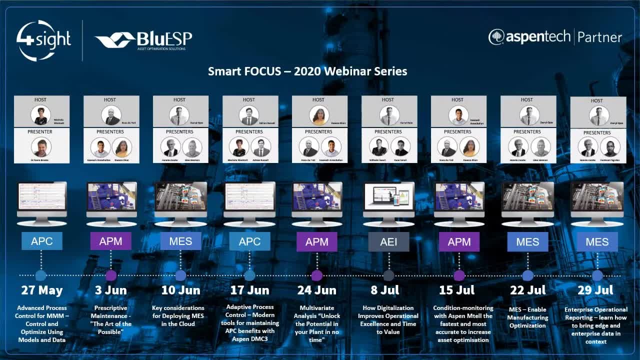 studies in South Africa, So really know their stuff and has been around and done lots of APC work. So you know we're going to talk a little bit more about that in just a few minutes. So, as you can see, we're going to talk a little bit more about the APC work for the last 15,. 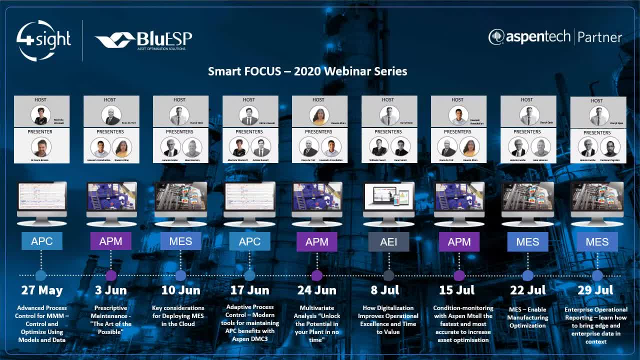 16 years of BlueSP, So we'll talk a lot about that. You can also see there's also for each one of these sessions we have two or three basically topics. So the next one up is asset performance management. This team has also just finished large entire projects- three. 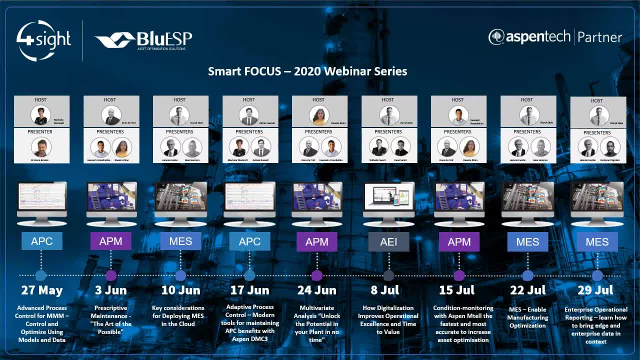 of them with mining companies in South Africa, in Botswana. They just engaged with one in Australia and busy with you know they're doing a lot of research on, you know, the various multivariate analysis proof of concepts right now, looking off the process: quality. 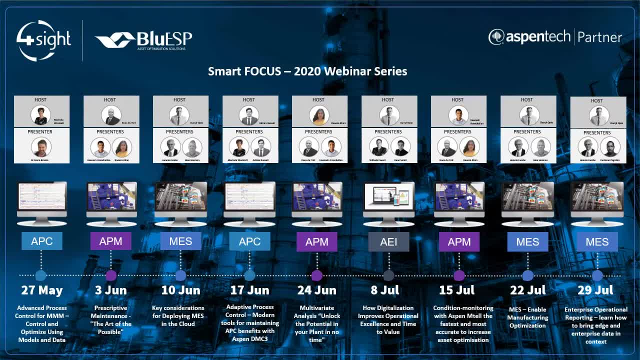 So they've got a lot to share as well. And then the last theme is manufacturing execution systems, So involved with projects in Asia. you know, just kicked off a very large metal accounting project in South Africa. looking at managed services projects related with 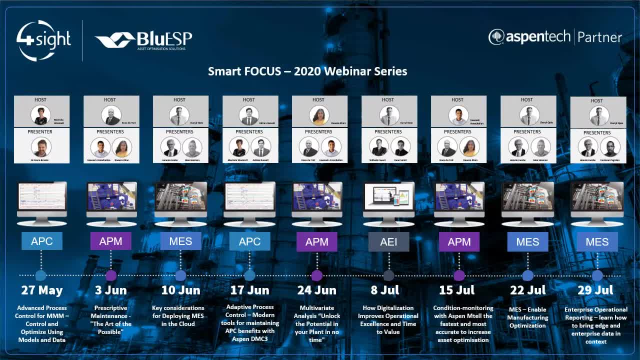 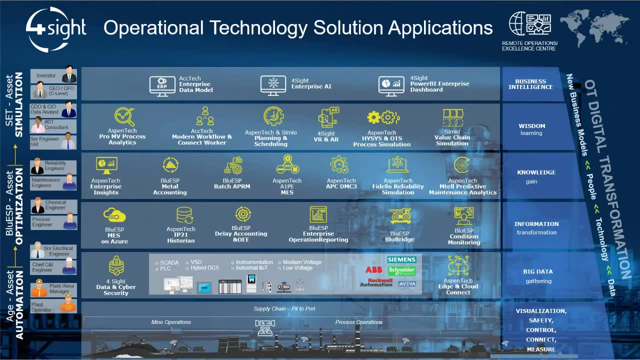 various large mining companies, also in South Africa and in the rest of the world. So we're looking at the next slide, Kevin. So really, what we wanted to try and do here is, you know, use the slide that just introduced you the intelligent technologies that we have in Foresight Now. so really, what we believe. 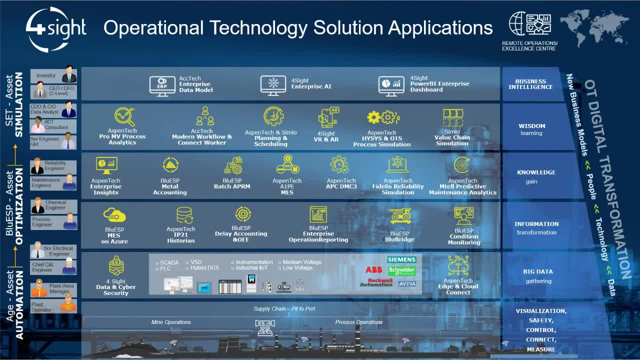 at Foresight is, if you take data and intelligent technologies, you get what we call an intelligent enterprise or enterprise 5.0, you know, and that's what we focus on. So if you look at this, it's a combination of data, technology and people you know and using those and bringing 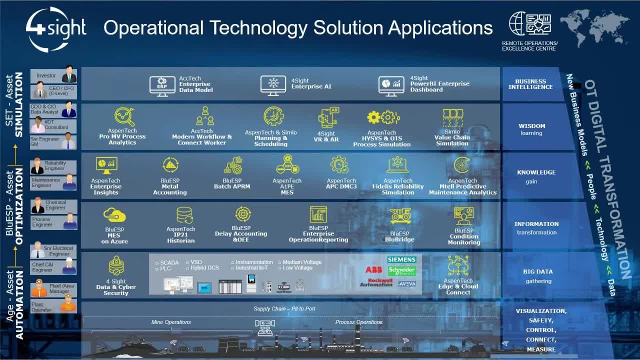 them together to bring new business models to the clients. you know, and most of these things today is happening in the cloud. So these intelligent technologies that we talk about as things like high IoT, so industrial internet of things, or artificial intelligent machine learning, deep learning, you know, adding that to existing software sets, that's. 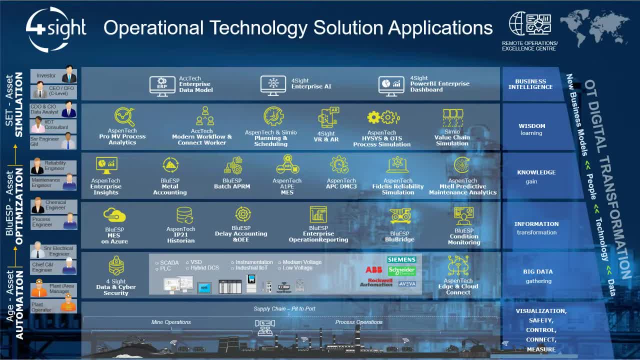 been around for 10 years. for 15 years is the norm of the day. That's what Asmodeeq focus a lot on right now. Advanced analytics is also. a lot of that type of work is being brought into the software enabled by the software multivariate analysis- to basically go through complex data. 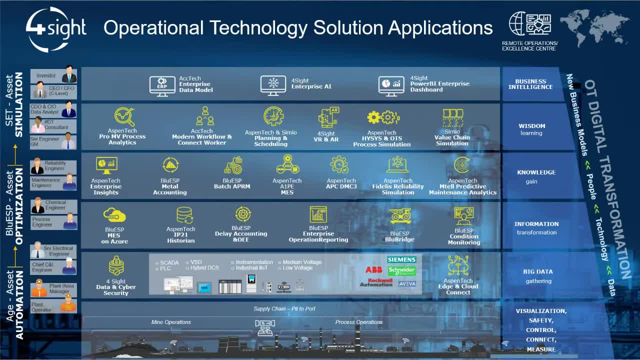 sets. simulation, planning and scheduling is quite core in there. improving the user experience with virtual reality and augmented reality tools And also all this information you know is being used to feed up into the ERP, the SAP environments, So that linking is. 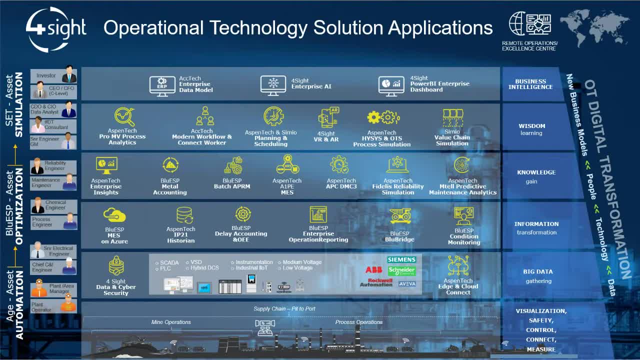 very important. So those are some of the intelligent technologies that we've applied on the screen. These technologies are brought to you by really three key subsidiaries in Foresight Group. So the first one is the Asset Automation Subsidiary 8 technology, and they focus on very much. 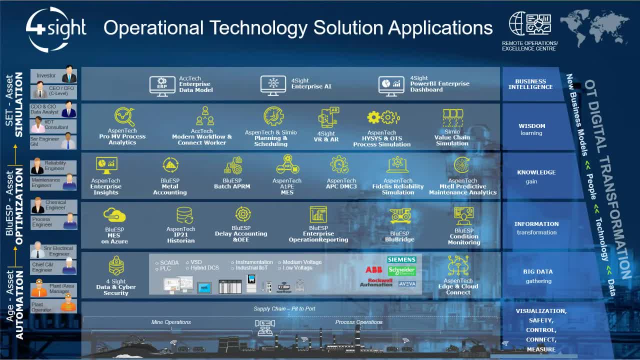 you know measuring the data, connecting to the data, controlling and making it safety. you know doing visualization systems. they are multi-vendors, so they work with the likes of ABB, Siemens, Schneider in automation projects and we work very, very close with them In the middle. you know, and really 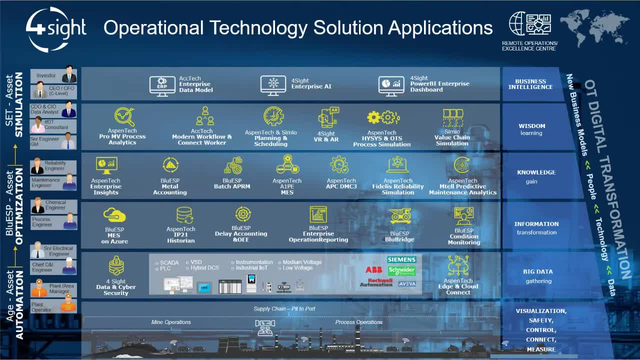 the, you know, is BlueSP. So BlueSP, as an Asmodeeq reseller and as an integration solution provider, is very much focused on transforming data into information, you know, bringing wisdom and knowledge and intelligence to the data. And then the third party is Simulation. 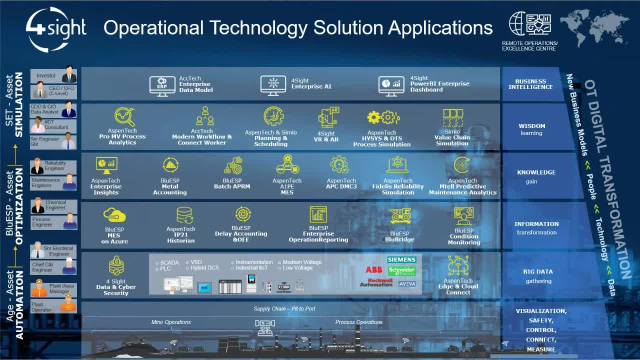 Engineering Technologies. a bunch of 20 people, Thank you. So we have 25 simulation engineers, industrial engineers, also in Johannesburg, very much focused on simulation of, you know, constrained simulation of mining processes and industrial processes, and also quite a lot of deep skills in planning and scheduling and assimilation. 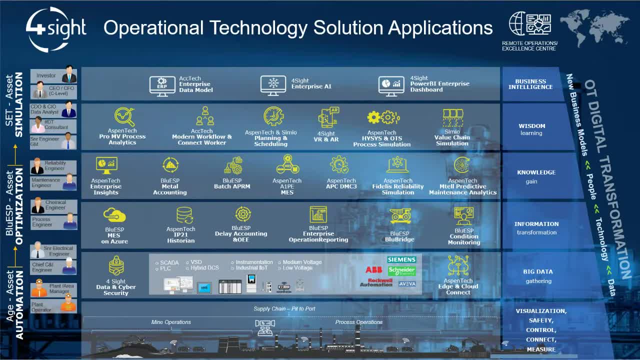 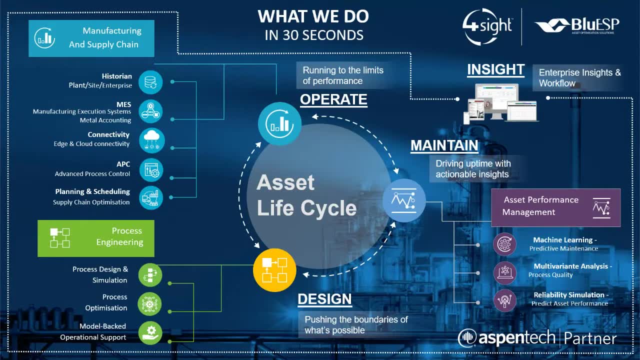 of that. So really those are the key subsidiaries that bring these technologies to you. So if we look now more detailed at BlueSP on the next slide please, So you know the way that we see BlueSP is really at our end. 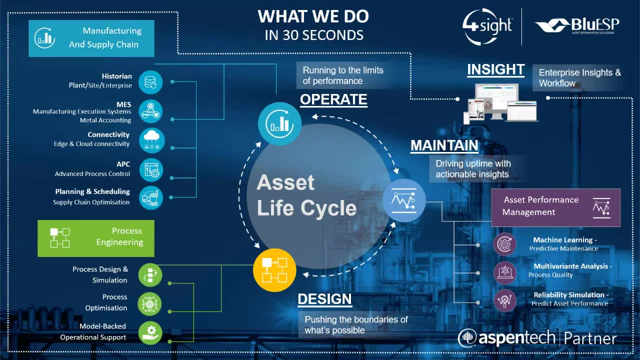 We see it as an agile and dynamic company. You know we basically use AspenTech as our road models to learn from them. to learn. you know they've got like more than 2,000, 2500 engineers that have been around for 37 years and then they develop some of the best. 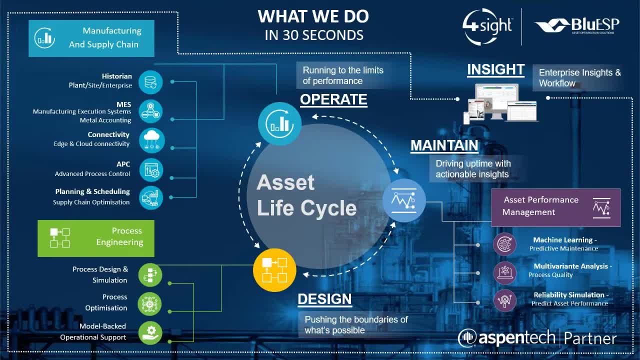 asset optimisation technologies out there today and we learn from them and we bring it to the local market. So some of these technologies- you know it's things like advanced embedded AI and their software. So more and more they take existing software. that's been proven. 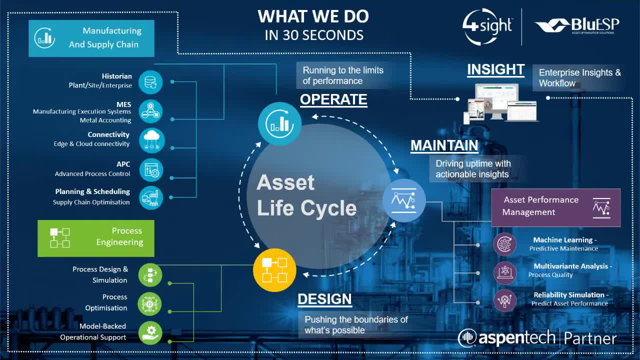 and test it and they bring AI machine learning to it, into the likes of advanced process control. we'll see during the course of these webinar series, or you know, hybrid models and machine learning like. example of that is the g-talk technology, where they use these technologies to orchestrate much bigger plant areas. Kevin might talk today about dynamic advanced control. 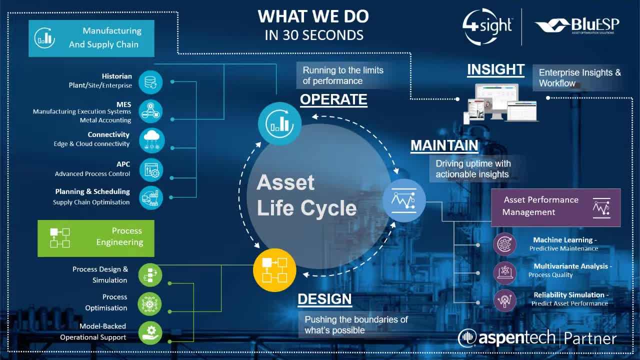 models and self-learning models, that you know that your plants and your control models don't auto-tunes itself and don't go out of sync. or you know things like artificial intelligence powered cognitive guidance systems to make you know the work experience much better. so various different things. so if we look at you know the way that Aspen Tech positions their 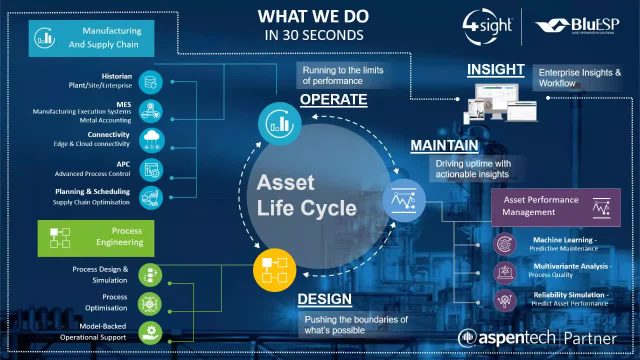 products. so the first set is the design sets of software, which you can see at the bottom there. so all about you know how do I simulate a new process, how do I design it, how do I cost it to its optimum and how do I build it. because if I'm going to build a new plant today, 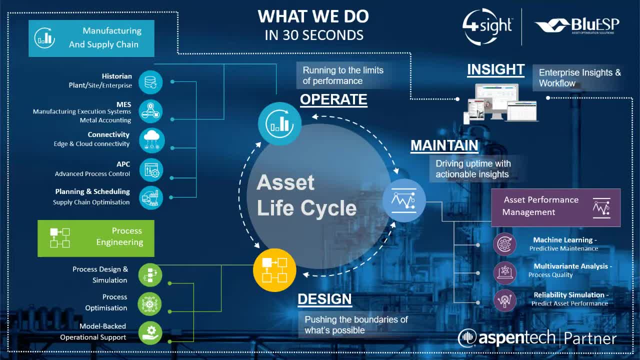 I want to build the best possible that I can do. we're not focusing too much on the design tools in this webinar, but there's a set of it. the next one is: how do I maintain and run my operational assets better, and so there's a whole set of tools, for example, related to predicting and preventing. 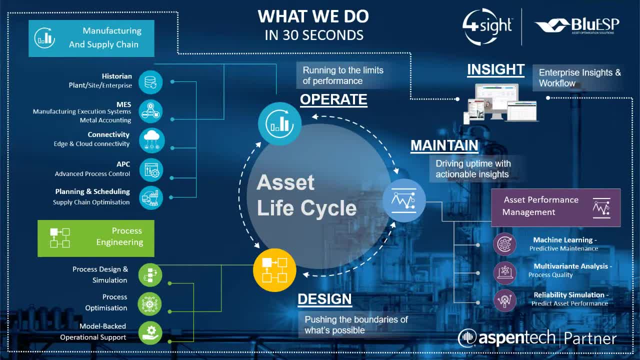 asset failures, the intel technologies which will come later in this webinar series. also things like predicting and preventing process quality failures, you know, and also simulation of maintenance and risk environments. so quite a lot of you know. you know tool sets there in this asset performance suite on the right hand side that basically adds: 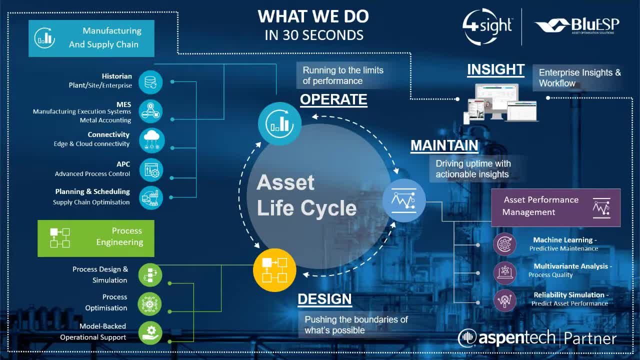 wisdom, knowledge and intelligence to data. in the area we're going to focus today is very much in the operational technology. so how do we run the plant better? we start by linking, aggregating the data, growing the data and basically, you know, transforming that data into information with 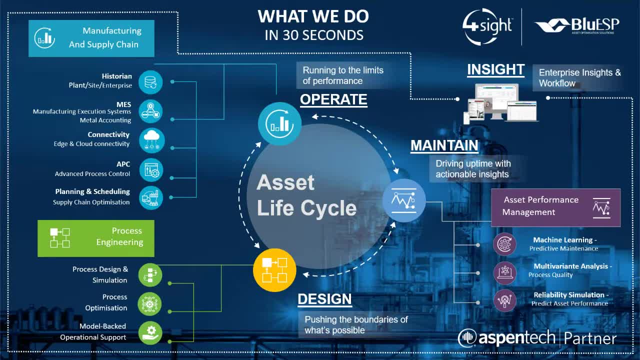 historian type systems. and and then you know next one is: is we? we would, for example, visualize the data in operational management and reporting system, mas systems that do mess, mass balancing or doing metal accounting solutions, or enterprise reporting. and then another key part is obviously advanced process control. so key focus is optimizing control of the modern 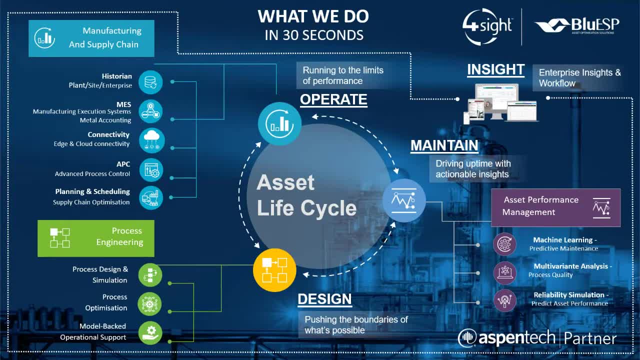 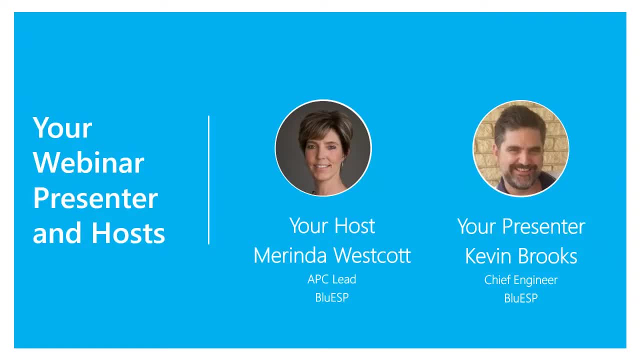 operation. so you know, that's the theme of today and, with no further ado, I'm going to ask you know marinda which? marinda westcott, which is the business unit leader of our advanced process control division at blue sp. which is the business unit leader of our advanced process control division at blue sp. 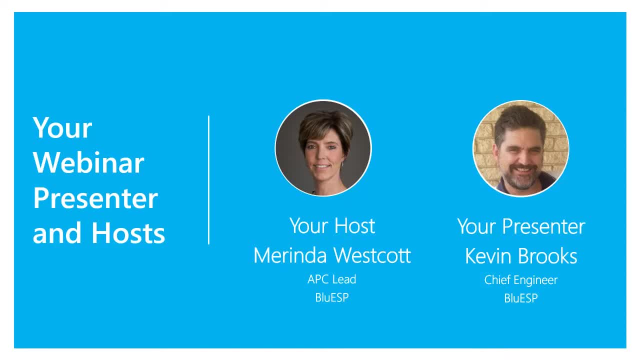 to just tell us a little bit about herself and also to to introduce the speaker of today, marinda, over to you. thank you for that introduction. good afternoon everyone, and thank you so much for taking the time to attend this webinar. as well as mentioned, I'm the APC business lead for APC. 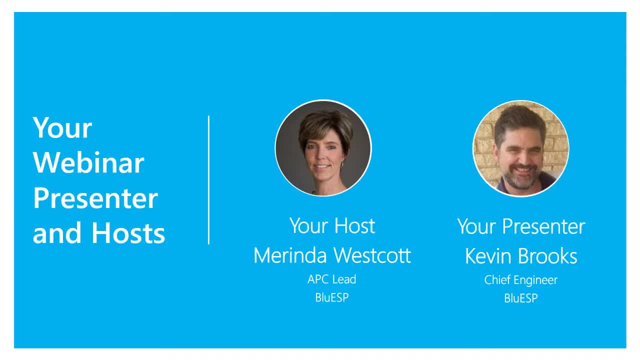 at blue sp. yeah, I've been involved in advanced process control for about 10 years. before joining blue sp, I was with sgs's advanced systems group where I did APC projects on mining sites mainly in africa, australia and canada. before that, I worked for impala platinum for 12 years in various 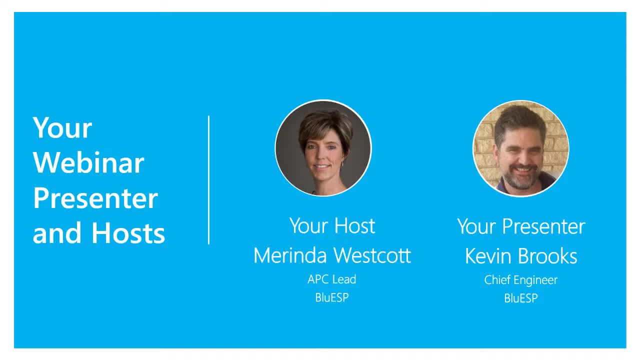 roles including process control, project management and plant process engineering. so today it's my great pleasure to introduce our speaker, dr kevin brooks. kevin has a bsc and phd degree in chemical engineering from the university of wits with waterfront, and he has over 30 years experience in advanced process control spanning many applications in both. 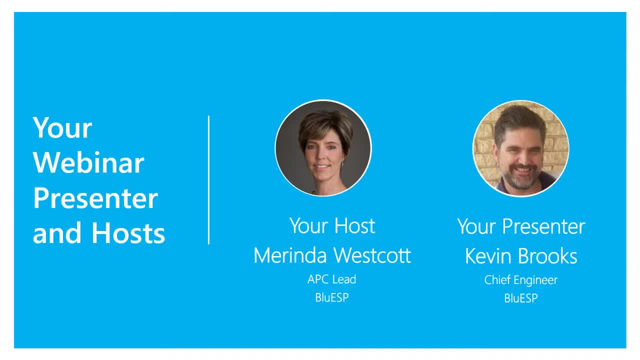 petrochemical and the mining industries. he joined blue sp in 2007, where he was an instrumental member of a team that introduced model predictive control into the mining industry. his most recent project was a year-long engagement with valet in canada. uh kevin is also very actively involved in the south african council for automation and control. 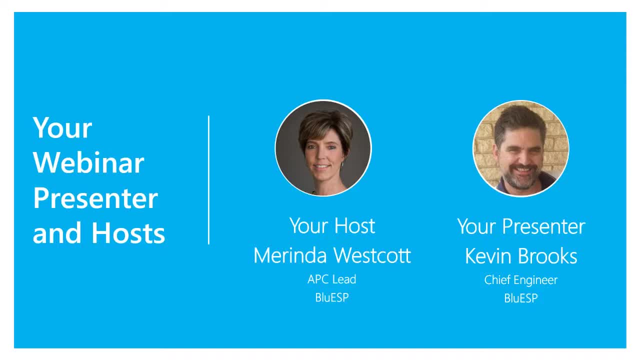 he was the president of this organization in 2013 and 2014.. most recently, 2019, he was appointed as a visiting adjunct professor at wits, where he's currently assisting with the teaching of process control. the title of kevin's presentation today is advanced process control for triple m control and. 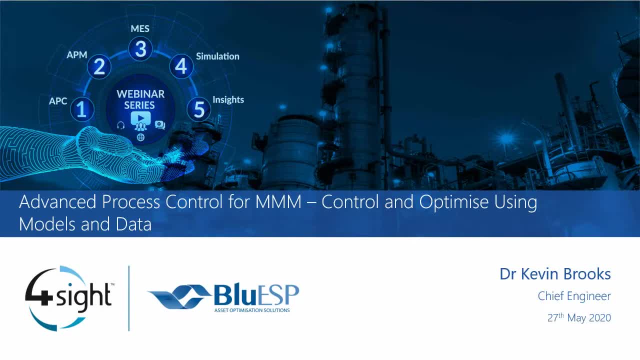 data with that. i'd like to thank kevin for sharing his extensive knowledge and experience with us today and over to you, kevin, thanks. thank you, miranda, thanks for the kind introduction and thank you everybody for taking some time out to to attend. we've been very pleased with. 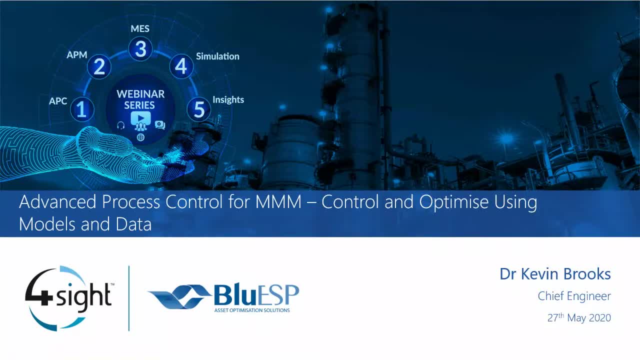 the attendance we've got. so today i want to talk about apc in triple m, and i guess i need to define what triple m is. it's metals, mining and minerals or in some different order, and i'm just going to say triple m. and really what i want to talk about is is how apc has become part and has. 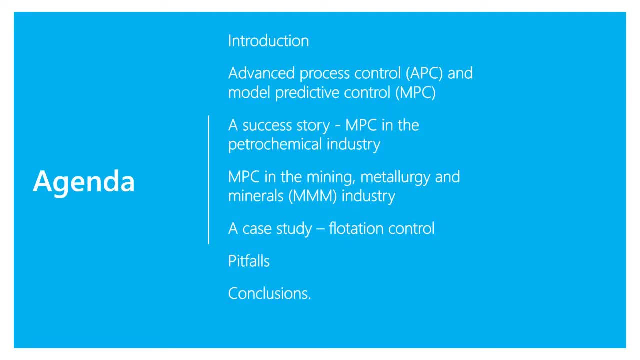 not become part of this world. so just to give you a bit of agenda for today, i'll introduce the subject and i'll i'll define some jargon, because i think it can be confusing when we talk about apc in triple m. so i'm going to talk about apc in triple m and i'm going to talk about apc in the. 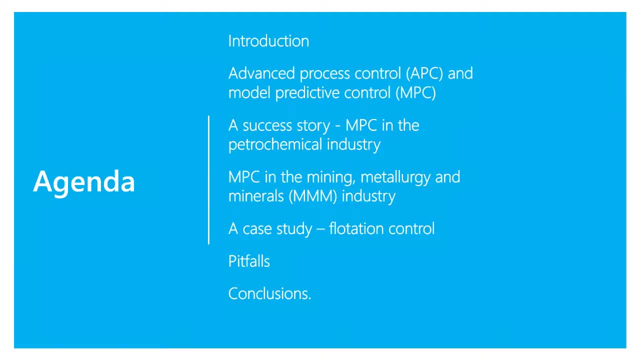 petrochem industry, not not because most of you are in petrochem, but i want to share its its success there and then move on to to its use in the triple m industries. i'm going to look at a case study to, to, to make the examples concrete, towards the end i'll give you some uh pitfalls. 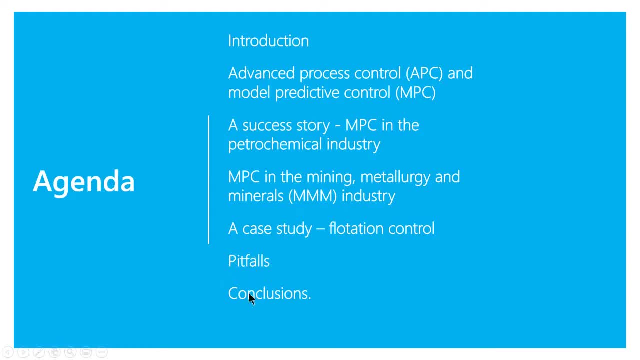 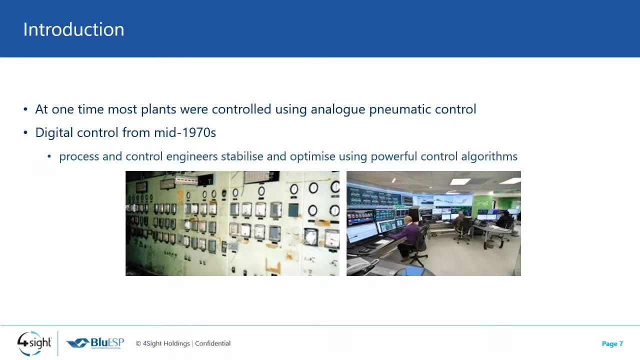 that you can fall into doing these, these projects and some conclusions, and there should be plenty of time for a question and answer session at the end. so, as an introduction, i doubt whether anyone here is old enough to remember the analog panels that we used to use to control plants, but those are. those are them on the left, lots of dials. 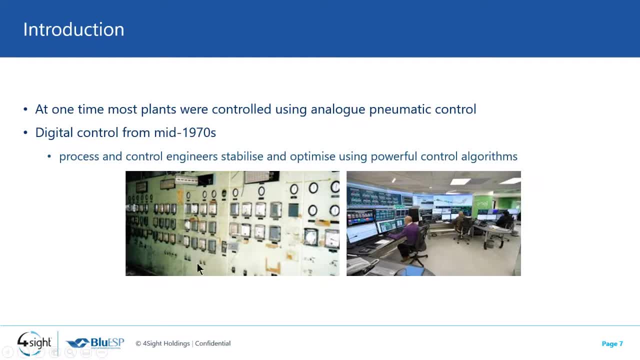 lots of strip charts with pins drawing on paper and red lights at the top often, which were alarms. and these, these control panels were analog. they used pneumatics, airflow to do pid loops and all sorts of clever stuff, but but that limited what we could do from a control perspective. 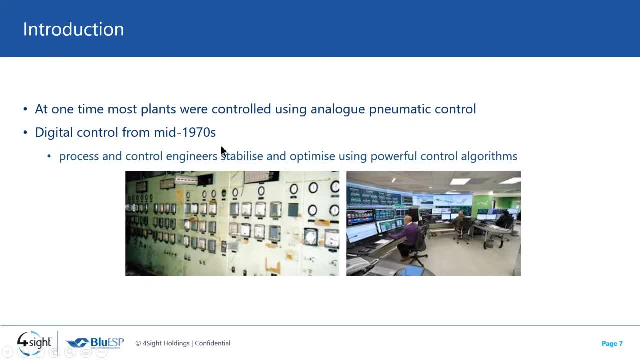 the introduction of the, the digital control in the mid 70s really led to the kind of control room we're all used to now: lots of screens, lots of computers and less dials and strip charts and. but from our point of view, what they really allow is for the use of powerful control algorithms. 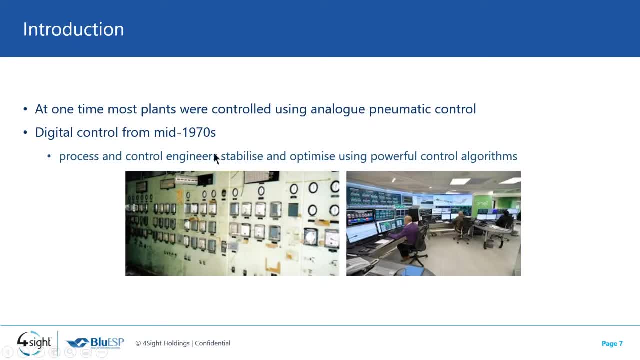 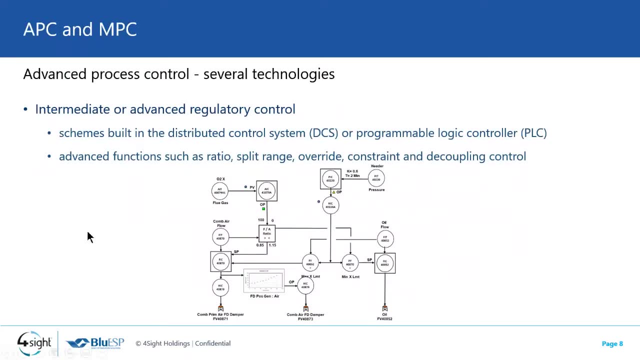 so if, if you've got computer programs running your control, you can do more sophisticated calculations. advanced process control isn't one technology, it's a set of technologies and people have different definitions of what they might be. i've picked out three or four here to talk about or to mention, and the first is 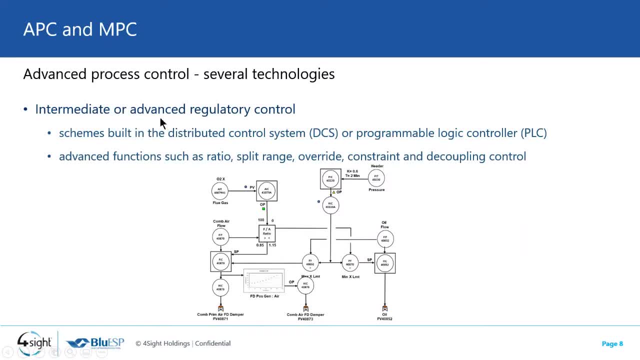 what used to be called intermediate regulatory control, or it's now sometimes called arc- advanced regulatory control- and typically these are schemes that you can build in your dcs or plc system. they are. they give you advanced functions like ratio control, a split range control, where you do. 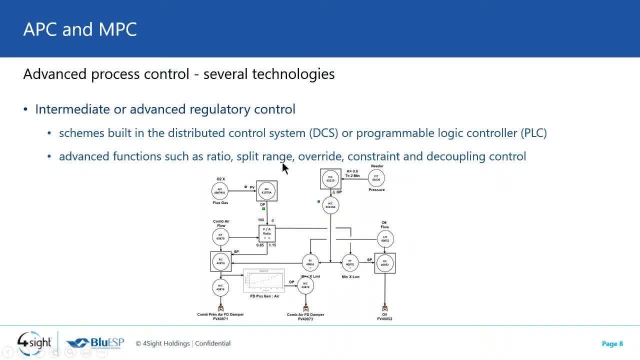 different things depending on whether you're above or below set point: overrides, where you normally control like that, but sometimes control in a different way: constraint control and decoupling control, which is kind of a first attempt to deal with multi-variable systems. i've just drawn one. 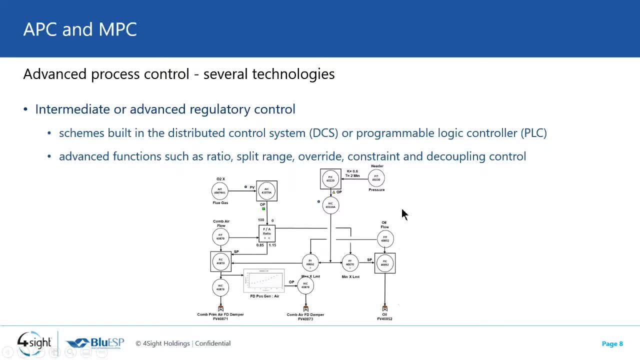 here which is a uh, advanced control, advanced regulatory control on a boiler. we've got a master pressure controller here which is writing down to various elements, and there's a a linearizer there, and so this, this has become quite standard, for instance for boiler control, and this would be an example of arc. 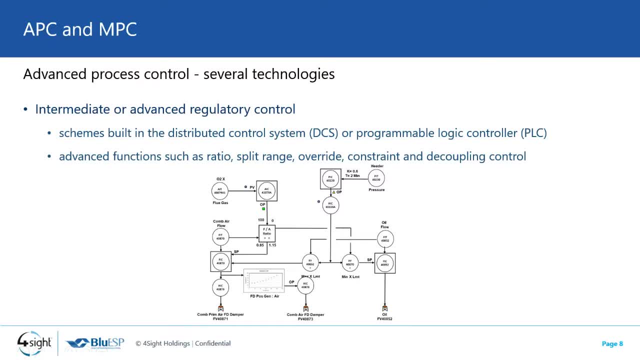 the problem with most, with some arcs or even most arcs, is that they are very well understood by the person who wrote them in the original and when that person leaves the company, no one knows how they can, how they work anymore, so they have a maintainability issue. 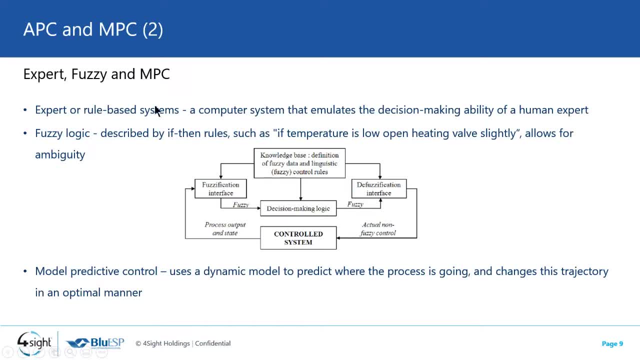 three other technologies include expert control, fuzzy control and mpc. so experts, or rule-based systems, are computer systems that emulate this decision-making ability of a human expert. so if you, if you have an expert who knows how to use a computer, you can use a computer to make decisions. 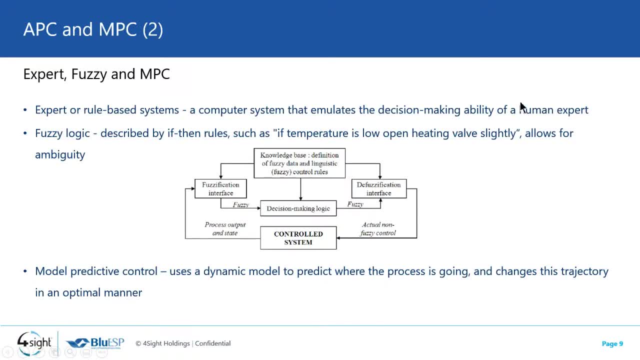 that emulate the decision-making ability of a human expert. so if you, if you have an expert who knows how to run your plant, why not just copy what they do in a computer program? that's what an expert or rule-based system does, and these are quite popular for some classes of control. of course, one has to 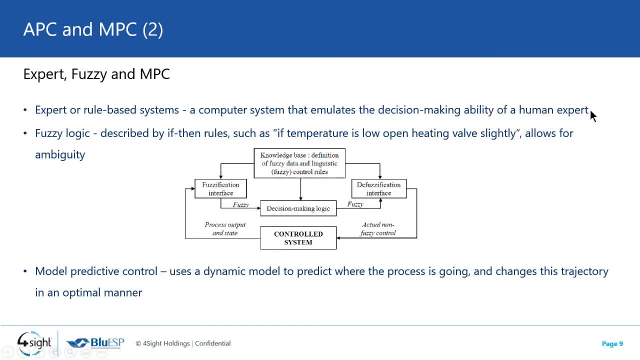 ask: why would we limit ourselves only to doing as as well as a person can do? maybe we can do, but better. fuzzy logic is also popular, described by: if, then rules, and with inputs that can be cold or very and very cold, so the inputs can be fuzzy. i've 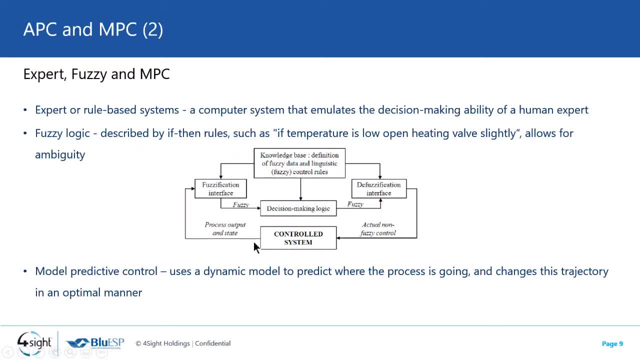 done a drawing here of a fuzzy system- became very popular in in the mining space at a time, i think, and and they certainly can do a job, i think- when we come to optimization, we find that these systems have limitations in terms of building the rules. we would need to optimize the 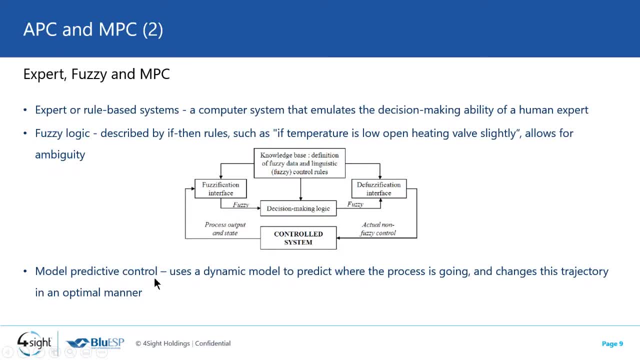 system. and then there's, finally, this model- predictive control- which is really what we're going to talk about today- which uses a dynamic model to predict where the process is going and then potentially changes the trajectory of the process in a way that is optimal and therefore makes money. 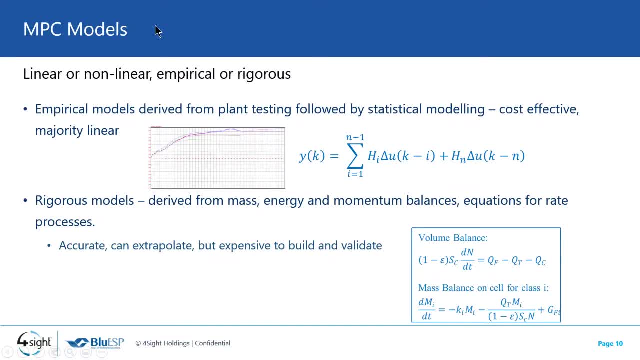 so if we're going to do model predictive control, we need models and we can classify these models that we that we use as linear or non-linear, empirical or rigorous. so, starting with empirical models, by that we mean that we find the models using data, we do a plant test or we go through historical data and we calculate some sort of statistical model. 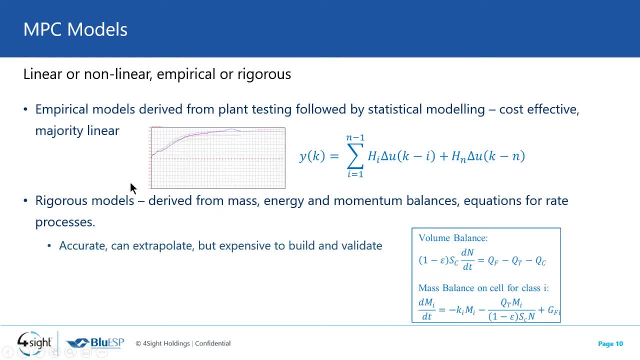 so there's there's. there's no physics behind this, it's all statistics, if you like. so this picture here is of what's called a step response, which is the response of one variable to a change in another over time. you can see that's fitted. so it's not fitted very well over there, but it's. this is a fit. 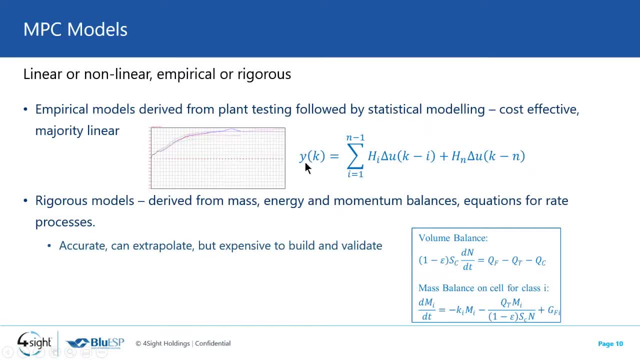 of data and we could express it in this difference equation form. this is the so-called f? r form. so this, these are, these models are empirical, um and validate, and in fact, to validate them we often need the data that we need to derive the empirical models. And here's a little example of two equations for the volume and mass of a material: 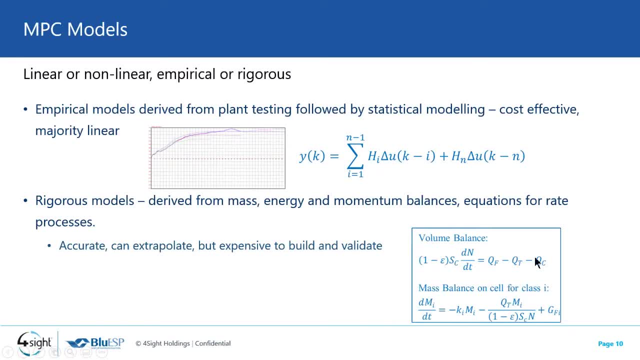 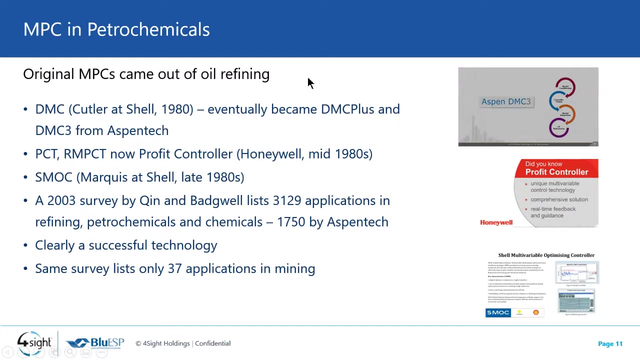 in a flotation cell. So we might start out writing equations like that. So what we find in practice is that the large majority of commercial MPC applications use linear empirical models, and that's from a cost saving perspective. A little bit of history about these MPCs. 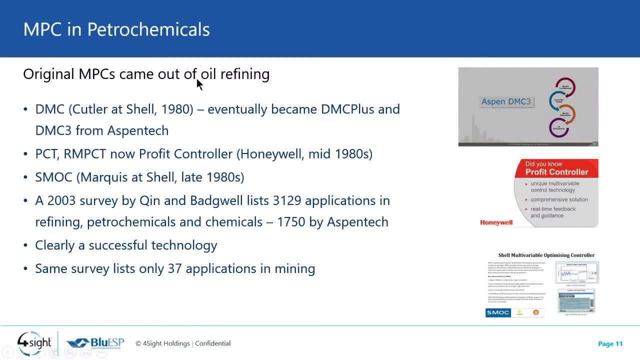 Originally they came out of the oil refining world mid 80s or early 80s. Cutler, who invented a formulation, if you like, of MPC called DMC, dynamic matrix control, which eventually became DMC plus and DMC3 from Aspen Tech. Unfortunately, Charlie Cutler died. 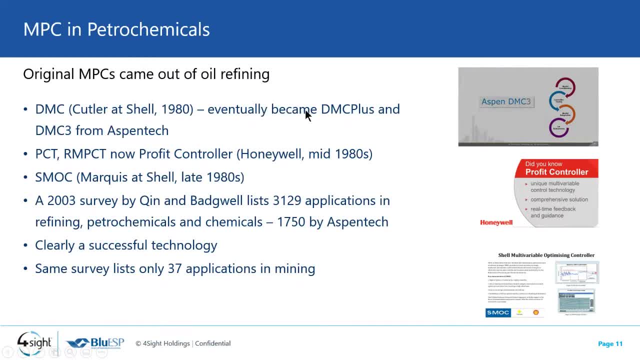 a couple of months ago. I've been told Around about the same time. some people from Honeywell and some companies that have been working on these MPCs have been working on these MPCs. So what we found is that Honeywell acquired, created a project called RNPCT, robust model. 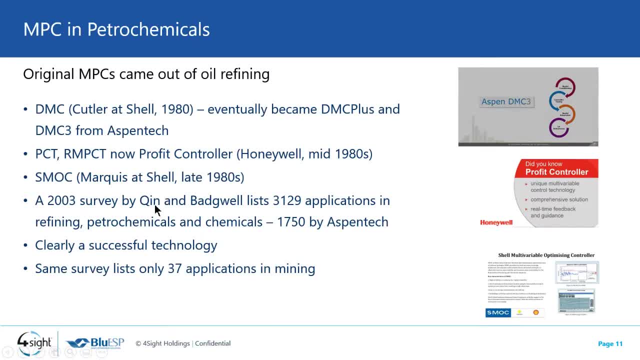 predictive control technology over here, and a different group at Shell, led by Pascal Marquis, developed a product called SMOC- I believe that stands for Shell Multivariable Optimizing Controller. Okay, and that's used. that's used a lot in Shell refineries, even currently, So it was an. 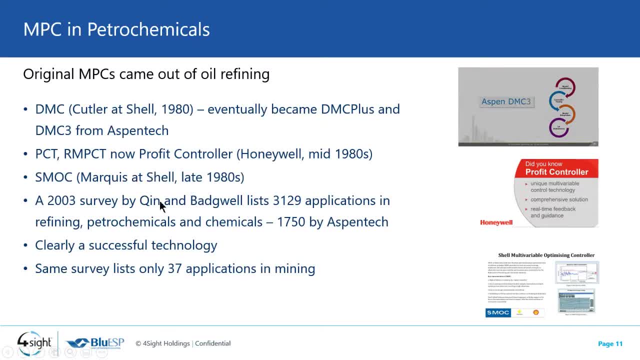 idea whose time had come. In 2003, Joe Chin and Thomas Badwell did a survey with the companies of MPC applications and they list three thousand odd applications in refining petrochemicals and chemicals, and more than half of those used Aspen Tech technology. So this is clearly a successful 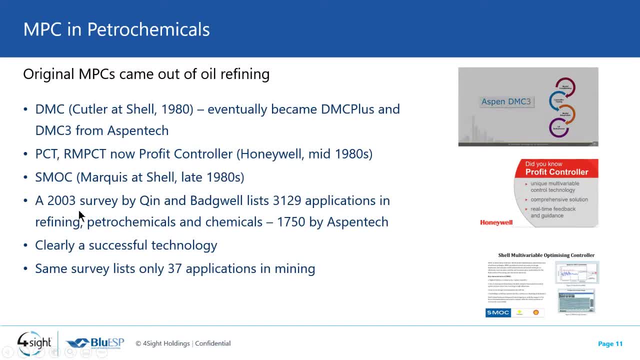 technology, and I think that's a great point, But the idea that you've got a company that's doing it. there are 3000 applications and that was 2003,. you can probably count on that being doubled by now In the oil refining game. nowadays, if you're going to build an oil refinery, 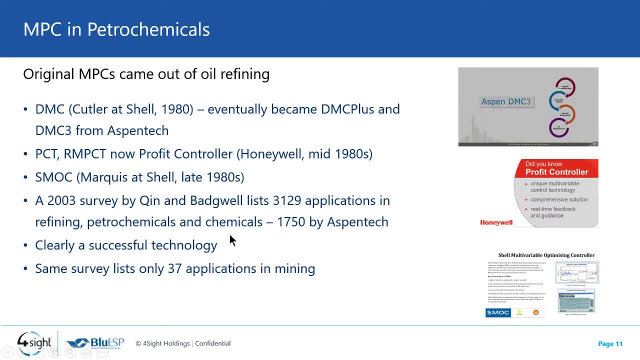 you would specify the MPC as part of the deliverables of the EPC. However, the 2003 survey by Chin and Badgewell only lists 37 applications in mining. So if we compare that to the amount of applications in Petrochem, it's very small. 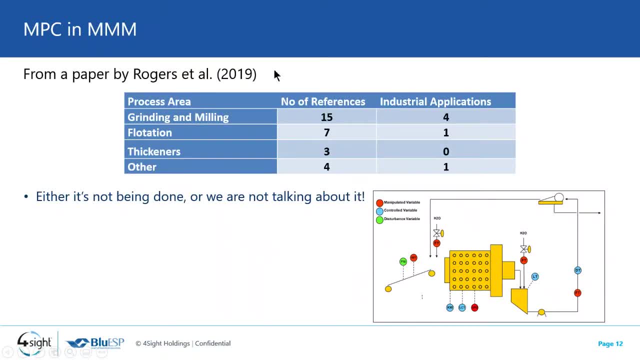 More recently, Rogers and co-workers looked at the literature for what's been published on MPC and they list a number of references in a number of processing areas. So if we compare that to the amount of applications in Petrochem, it's very small. 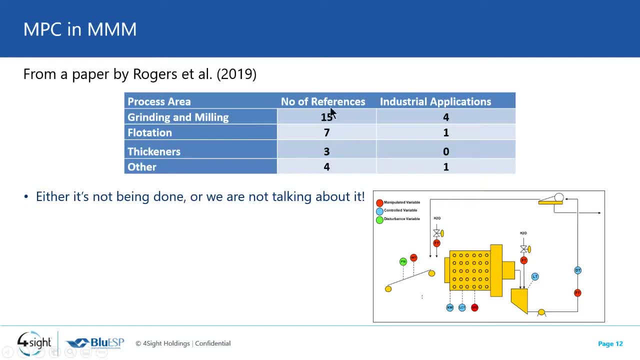 So if we compare that to the amount of applications in Petrochem, it's very small And they're all very interesting. The trouble is only six of them in total are industrial applications. So something strange, because either we're not doing MPC in Triple M or we're not talking about 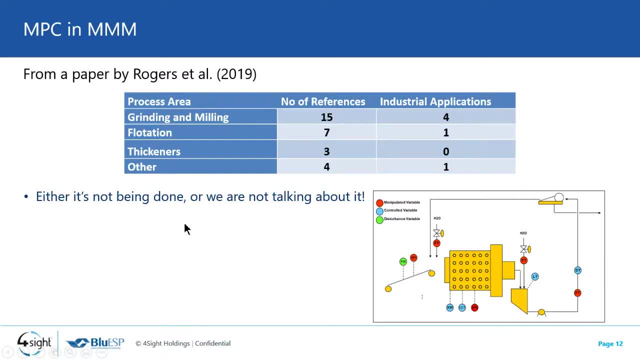 it, And I think it's a bit of both: We're not doing as much as we could to improve operations using these technologies, And then the ones we have done we're not publishing. So there's room for improvement here, And here's a little picture some of you may recognize. 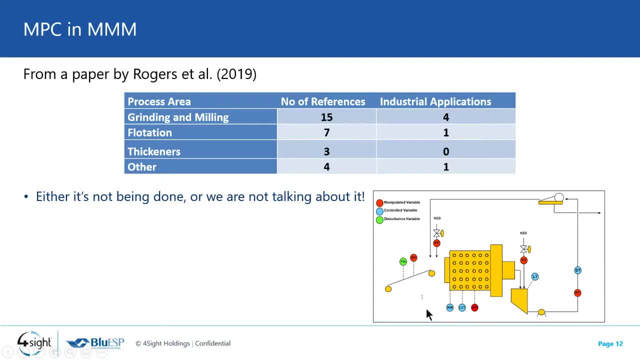 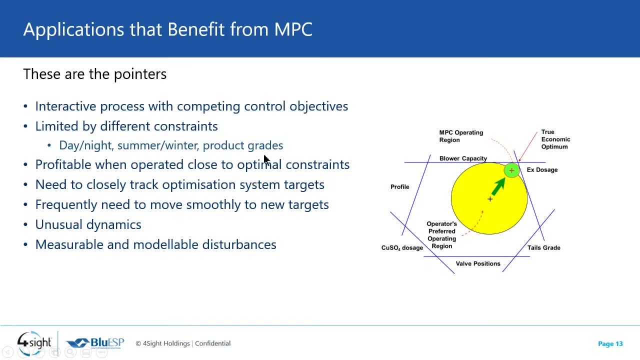 of a grinding mill and how we would at least specify the inputs and outputs for it. So clearly we're not going to do MPC because it's a cool technology and we like building models. We need pointers to what kind of processes would benefit and what are the financial benefits. 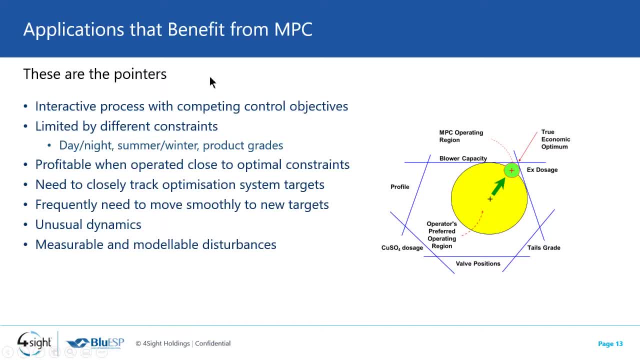 So because MPC is model based, it enhances the efficiency of the process. So because MPC is model based, it enhances the efficiency of the process, Inherently handles the interactions within systems. So a lot of the processes we deal with are interactive. 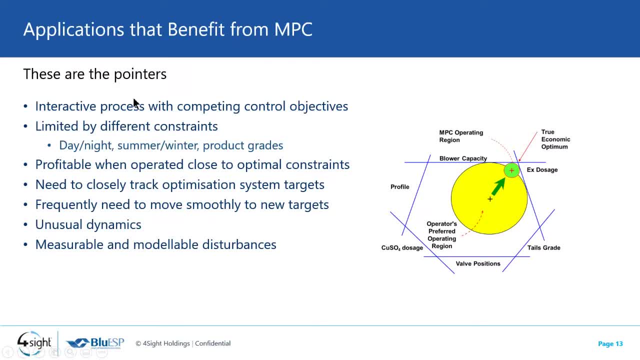 If we increase the feed to a mill more than one thing changes. We may have to make other changes to compensate for that. So there, the model predictive technology helps greatly In some cases. we're limited by different constraints at different times. 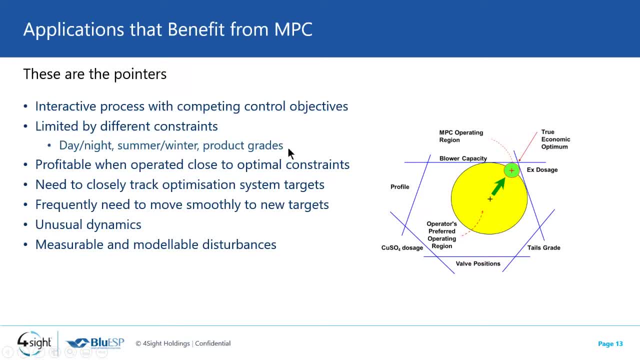 It could be day, night, summer, winter or product grades, So we may have to change grades. In that case, you want a flexible control system. This third point is really very important If your system makes more money when it's operating close to constraints. 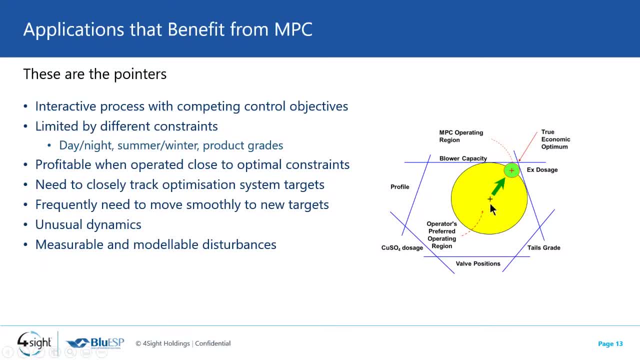 it is a good candidate for MPC because what the MPC does is it takes the operating point that we have now somewhere over here in the middle within the operator's comfort zones, and pushes towards the operator's discomfort zone where the operator won't operate And if in that pushing we make money. 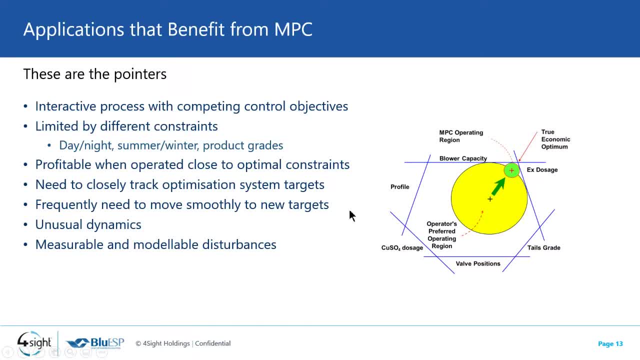 then we can make that money consistently. So if we need to track optimization targets, then MPC is a good technology. If we need to move to new targets, this perhaps is less important in Triple M, but maybe if you're running a polymer plant it's very important. 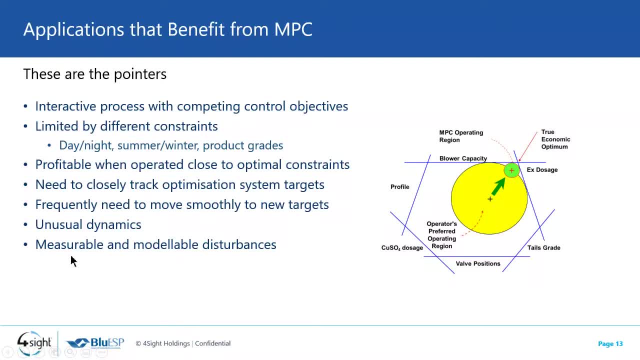 If you have unusual dynamics and if you can measure and model the disturbances. So this we do see in Triple M. We can measure grades coming into a mill or a flotation plant and we can get models for how those affect that plant And in that case we can do some very 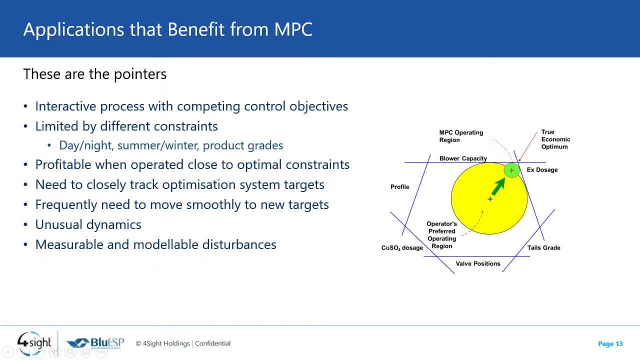 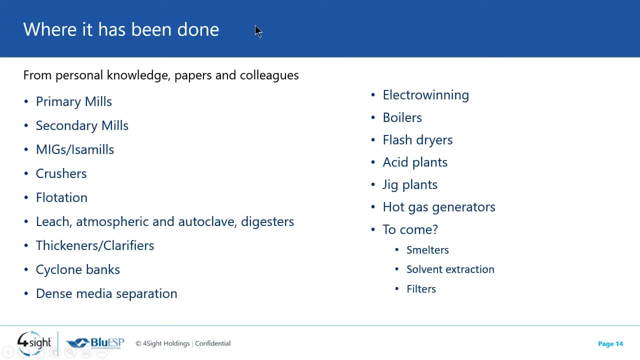 powerful proactive control of the system. So, despite the paper by Rogers, I thought I'd put together a list of where I know MPC has been done in Triple M, either where we've done it or where colleagues have done it or I've just heard. 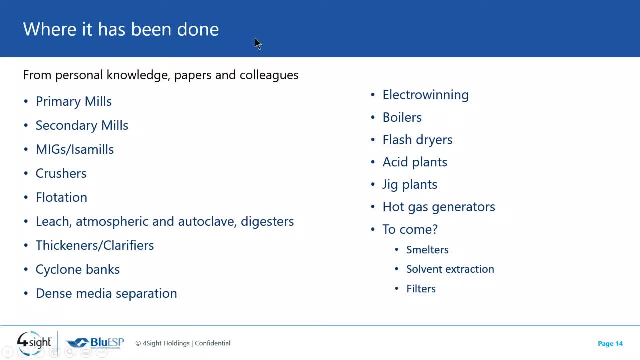 about it And it is a large list. Mills in particular, Primary, Secondary, AG, SAG, Iser Mills, Crushers, Flotation, which I'm going to talk about later, Leaching some work I've been doing recently and some work I know that was done at Alcoa. Thickness and clarifiers have been done. 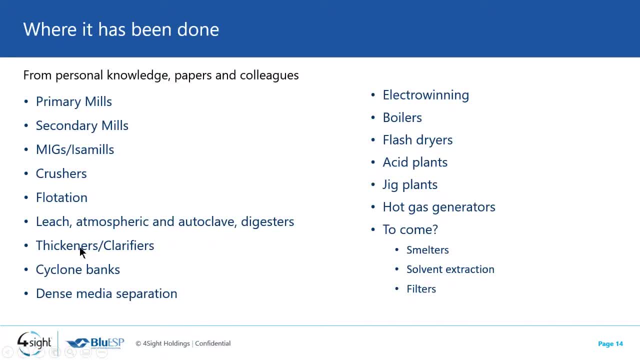 We've done cyclone banks. There has been some look at dense media separation- not as much as I would like, but I think it's really important. We've done a lot of analysis of the different types of processes. We've done electrowinning. Boilers are interesting because you shouldn't ignore the utilities. on. 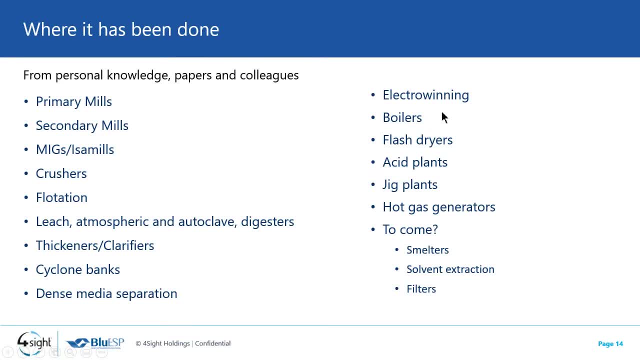 your plant. This might be low hanging fruit for quick wins on benefits: Flash dryers, acid plants, jig plants, hot gas generators And ones that I don't know so much about but which I'm quite I think will come, are smelters, solvent extraction. 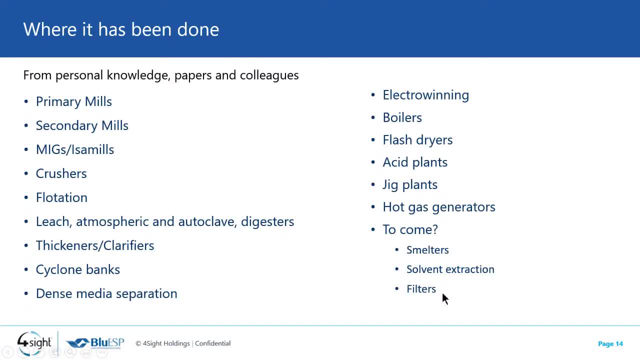 and other things like that, And although it may seem like a simple unit operation, it looks to me like there are cases where filters could benefit from this technology. So this is a wide range of unit operations that we have and could look at with MPC. 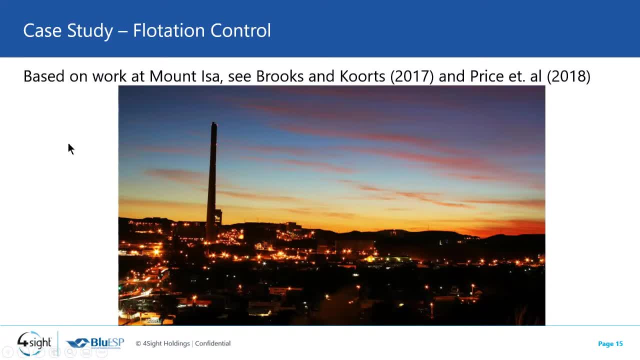 So for a case study, we're going to look at work done by this group in Mount Isa. Mount Isa is in Queensland, Australia. It's a very interesting site geologically because it has one, a vein of which is lead and zinc and another vein which is copper, And so there are two processing plants on. 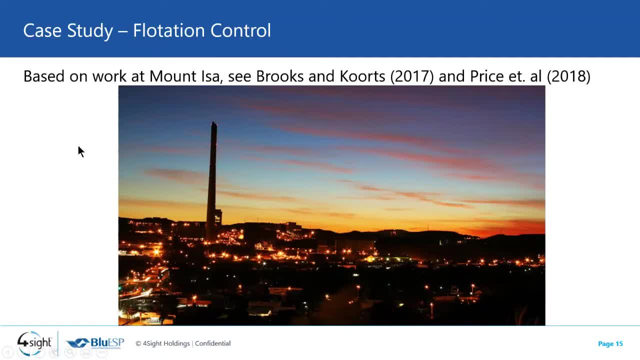 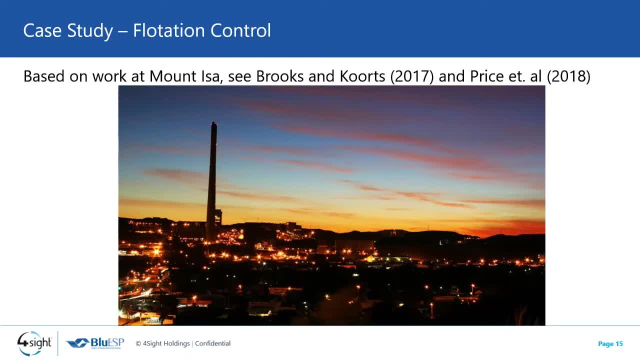 doing two different processes or making two different materials. It's very famous for its very tall stack, because there's a lead smelter on site, and so they put the effluents up high. The work I'm going to talk about there are some. 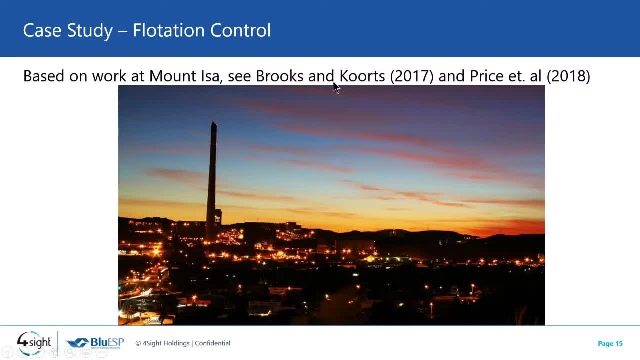 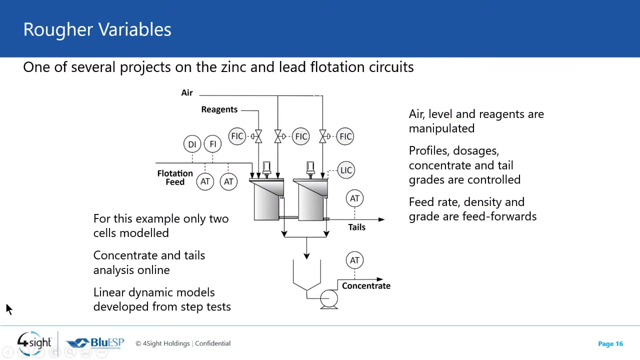 publications. Myself and Ryan Courts have written a paper and Adam Price, who is with Glencore, and some of his colleagues and me, wrote another paper which is available, And we did a number of projects on flotation, both zinc and lead circuits, And I'm just 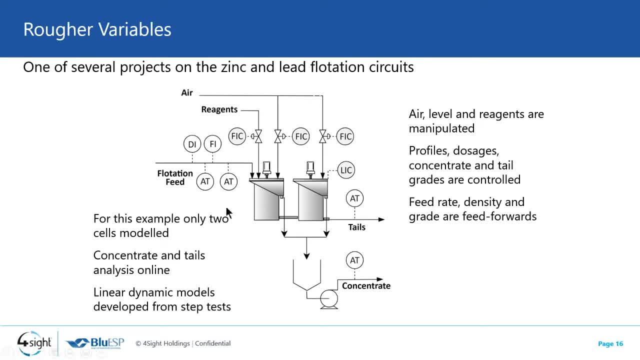 going to take as an example of what we did two cells. Obviously we had more than two cells, but just to make it easier to understand. So we're going to look at how we would model two cells And in our particular sort of model example, which is very much like the real example. 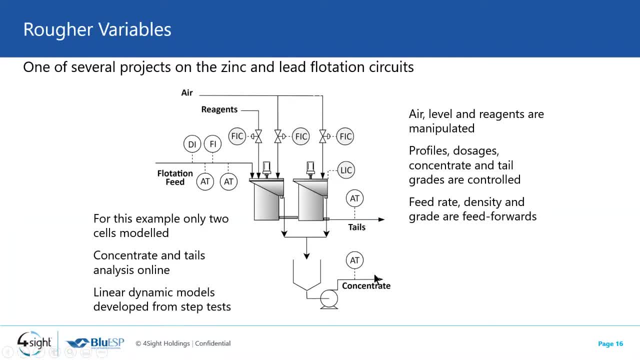 the concentrates and the tails. their grades are measured online. In this particular application, they're measured by XRF And we're going to show how we develop linear dynamic models from step testing. To understand the system, we need to know what are the inputs and the outputs. 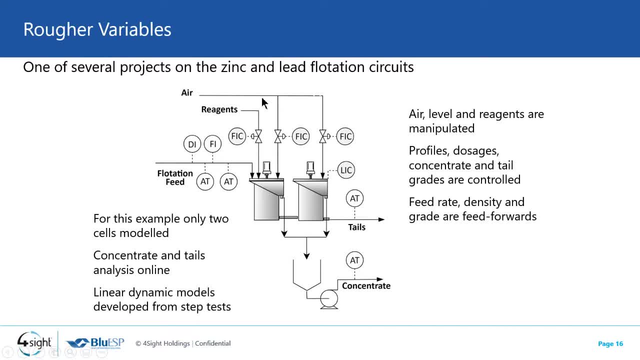 And for this particular system, the airflow to the two cells are inputs. We can independently change those, as are the reagents Over here. we can independently change those And the level. there's only one level between the two cells And we can change that with the dart valve. 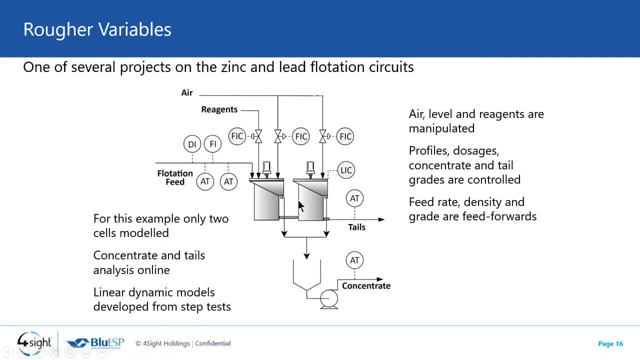 The things we are controlling are the profiles, for instance, the difference in air, the dosages of the reagents and, obviously, the concentrate and tail grades. What are our disturbances? What are the things that we would where if there is a change? 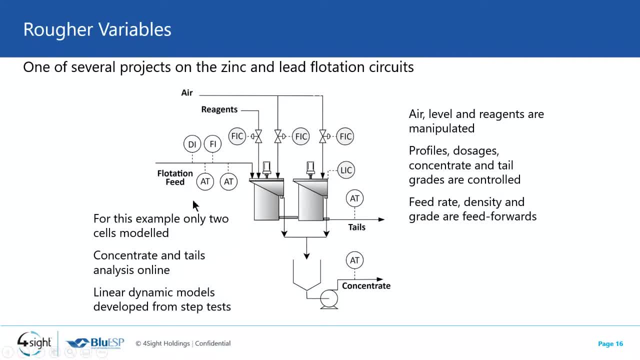 we would like to reject that change. Well, those are all over here on the feed side. So that's the feed rate, feed density and the feed compositions, which are also measured. Okay, So how do we do this? Well, what we do is we go off and do a. 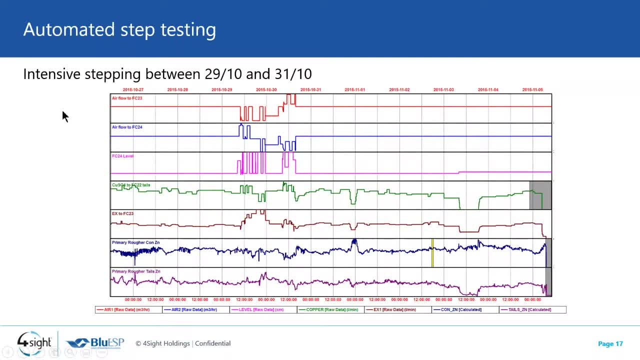 series of step tests. Okay, And what I've shown here is a period of intensive step testing of the air and the level and the copper sulfate, which, if I remember correctly, is the collector, and the X, which is the sodium ethyl xanthate, which is the depressant. I may have those two. 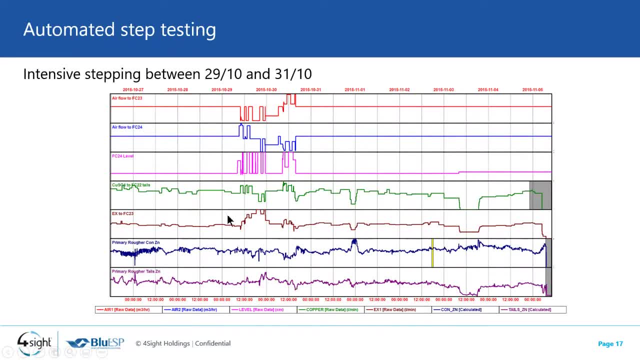 the wrong way around And over this period- here you can see- we are injecting steps into those inputs. So we're doing a planned experiment where we're moving this. This, in fact, was done by the computer. Okay, Historically we used to do these things manually. We still. 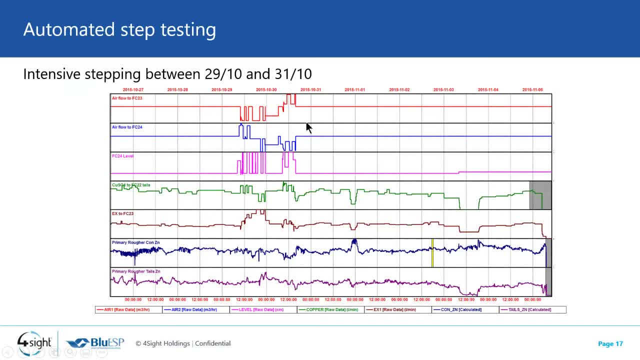 sometimes do it at the early part of the project, But afterwards we've got tools now that will do it automatically, And I've shown just two outputs here. So these are the primary rafficons- zinc moving around presumably as a result of all these moves we're making here, And the same 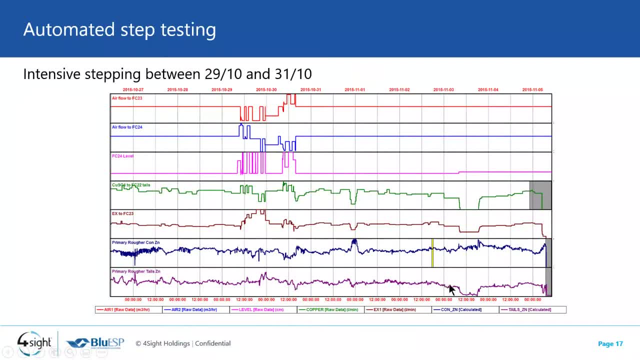 with the primary rafficons: tail zinc. Those are moving around. Something went wrong there. We'd have to get rid of that data And the reason I've shown more data is just to show that some of the data that was not where we. 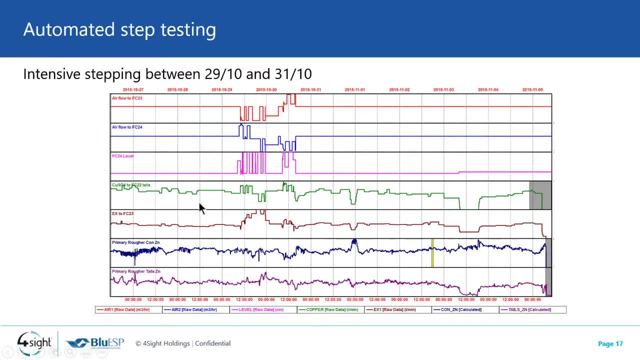 weren't stepping. these were the ones that were moving around, And the reason I've shown more data is just to show that some of the data that was not where we weren't stepping these variables can still be used, because the operators were presumably moving some stuff around here as well. 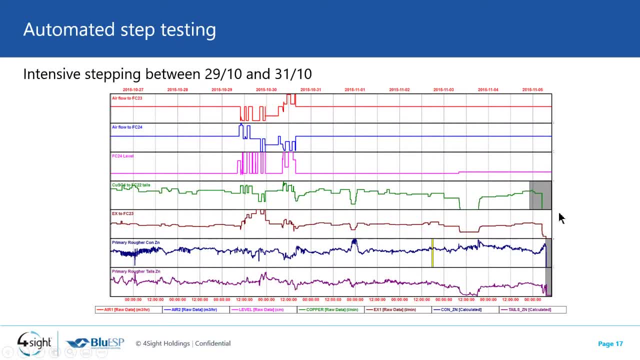 Okay, So this is the AI plot, if you like. We never used to call it that because we didn't know what AI was, But this is the part where we take this data and we attempt to turn it into models, And the models look like this. These are called unit steps. 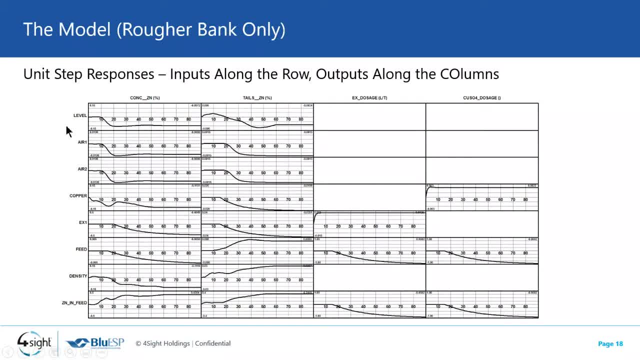 The unit refers to the fact that they are drawn for a step of one in the input. So, for instance, this model here is the response of the concentrate zinc to a change of one, presumably percent in the level and with over a 90 minute time period. 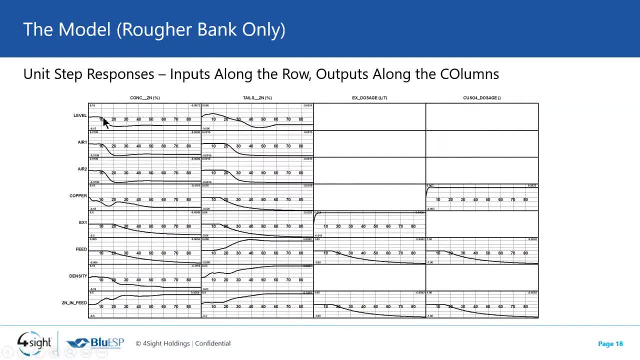 So what do we see happens? Well, nothing happens. for 10 minutes. There's a delay, Then there's a reasonably sharp drop and then the zinc stays reasonably constant. Some other models down here where the density goes up and this causes the tail zinc to go up. 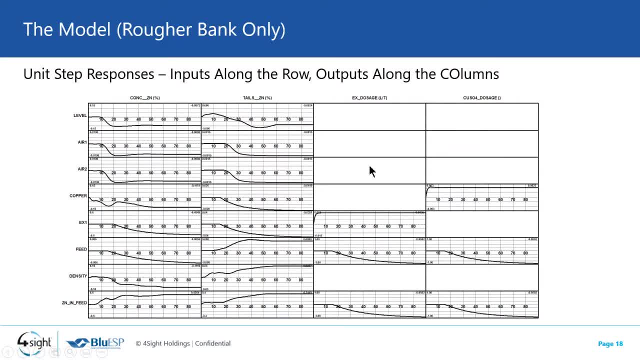 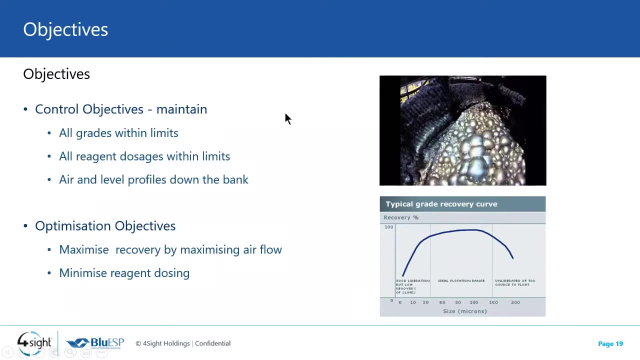 So these are statistical models, they're FITs, And the more data we have, the better the FIT. And we've got very sophisticated tools. What are we doing now for doing this, fitting in the Aspen-Tex ainda software? What can we do with these? Well, we have to define our control objectives. So for this process, 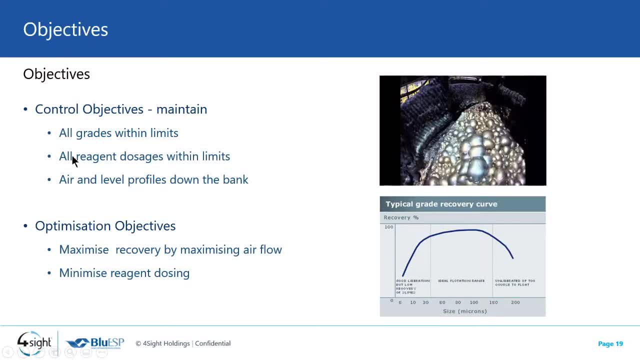 we want all grades within limits. We want reagent dosages within limits. Ideally the system should know, should find the reagent dosages So that we can define the control objectives. But generally the metallurgist needs a range of dosages within limits. 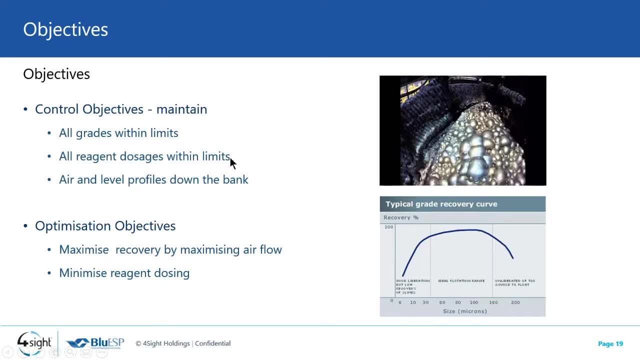 paleontologists do want to say: well, even if you want to reduce the dosage below 0.1, I'm not going to let that happen. So we have to keep dosages within limits. and then we like to maintain a particular air and level profile down the bank, And then, for optimization, we maximize recovery. 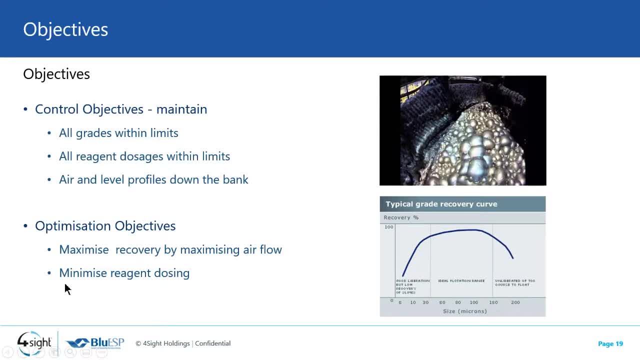 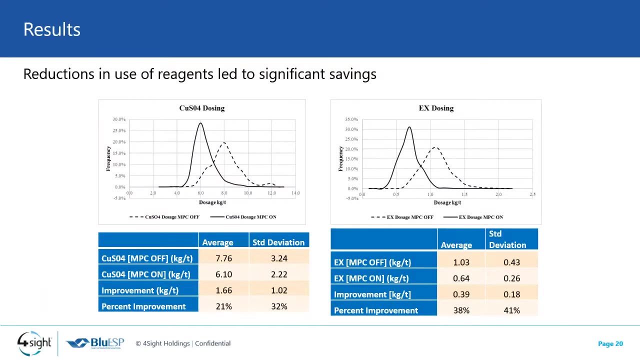 by maximizing airflow and at the same time, we minimize reagent dosing to save money on chemicals. What do the results look like? Well, these are some results from paper by Brooks and Quartz, and what we're drawing here are histograms of the dosages of the two chemicals and the dotted line is the histogram of frequency distribution. 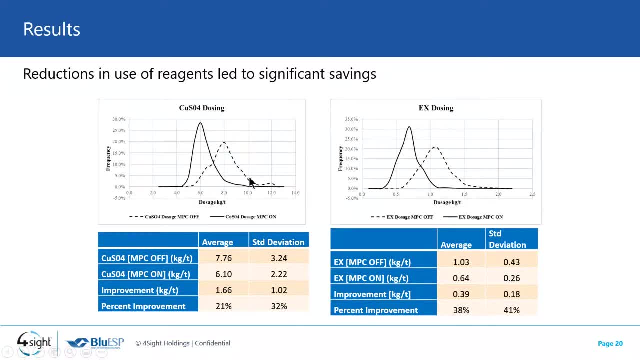 before we even start sampling the dosages did the APC, MPC and the solid is after, And you can see very clearly here that we have a sharper distribution, which means we're controlling better, and we've moved the average significantly down, in this case from 7.8 to 6.1.. That's a 20% improvement. That translates: 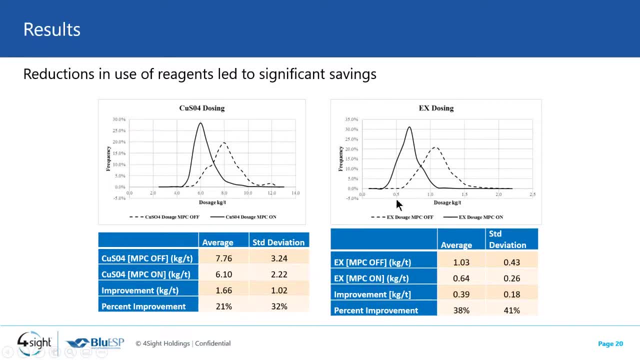 straight into the bottom line. Similarly, with the ethylxanthate it's even more: 38%. So the aims of the project were very well met and this is subject to always being within grade constraints and recovery constraints, So this is a very visual way of looking at. 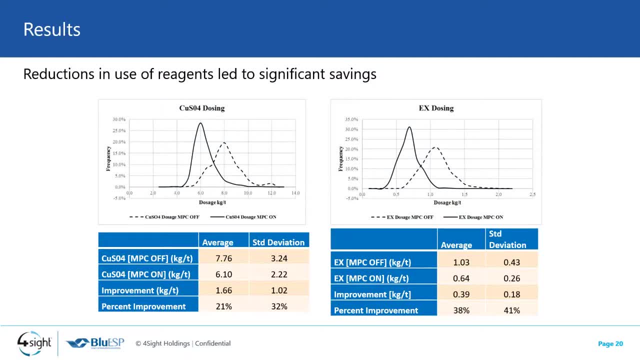 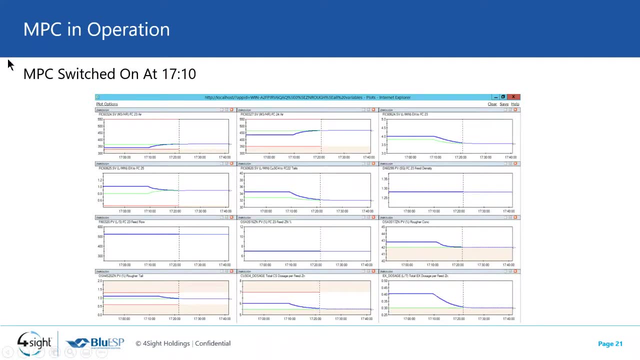 the results from these sorts of projects. Here's just an example. Here's an example of what might happen when you switch an MPC on in the evening. So these are just time plots, with the dotted line being now and everything to the right of the dotted. 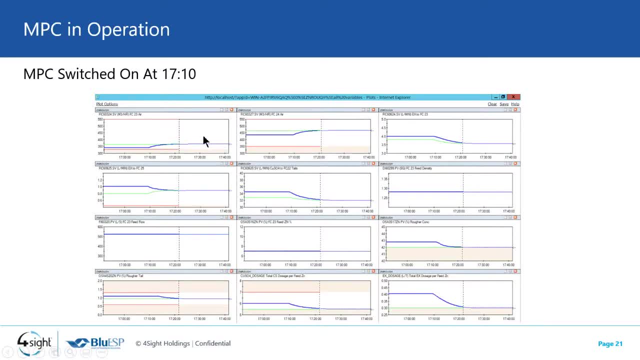 line is a future prediction. It's always taken by the fact that, in fact, an MPC is rarely the only place in a plant where you can visually see at least some idea of what's going to happen in the future. So this is about a couple. 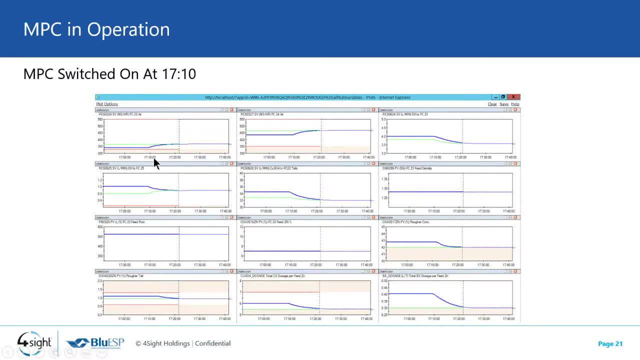 of hours into the future here. So at this point here, we switched on the MPC. It picked up the air, It lowered the ethylxanthate here and here and the copper sulfate. These are the disturbances which we've left constant in this simulation, And the result is that 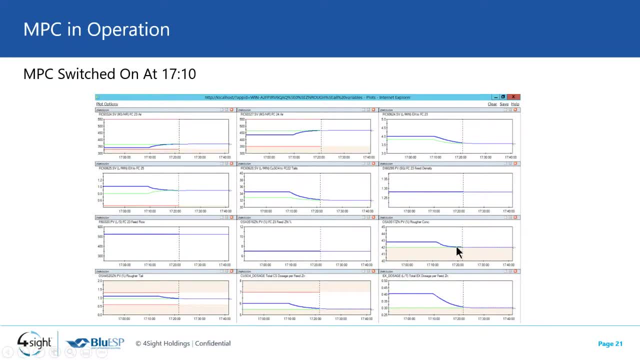 the result is: the raffa came down, but it didn't come down below its low limit. Raffa tails came down a bit, which is recovery, and then the dosages came down. So this is a simulation, but it does show how you can make money using coordinated moves while maintaining. 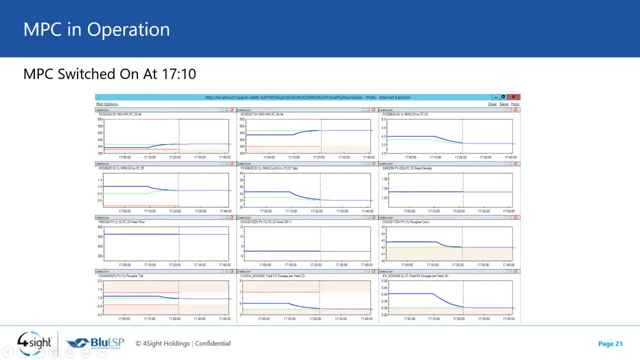 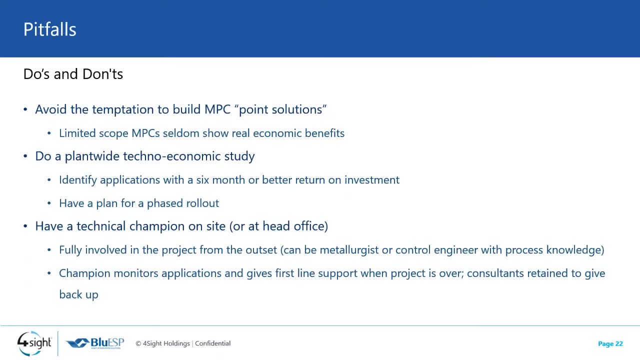 within the constraints of the system. Okay, I did say I'd I'd mentioned some pitfalls. The first one is I've seen MPCs used and other control systems used to solve very point problems, very small scope problems. I would say: don't do that. 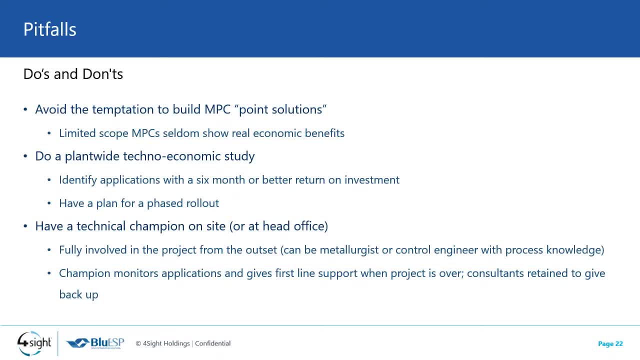 Have decent scope on your controllers, because then they will show real economic benefits. Do do a plant-wide techno-economic study. This is something We have pushed for and have done for a number of clients, and we used them to identify applications with a six-month or better return on investment, which is great. to have a phased rollout and. 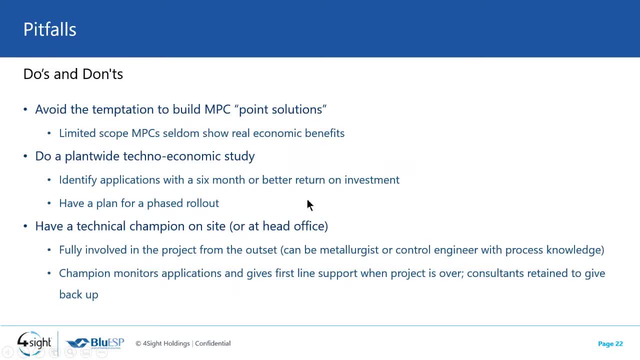 this means that the programme becomes self funding, because the first project will pay for the subsequent projects And you may have to pay for this study, but it's worth it. and then have a technical champion on-site to solve problems. Okay, Thank you. 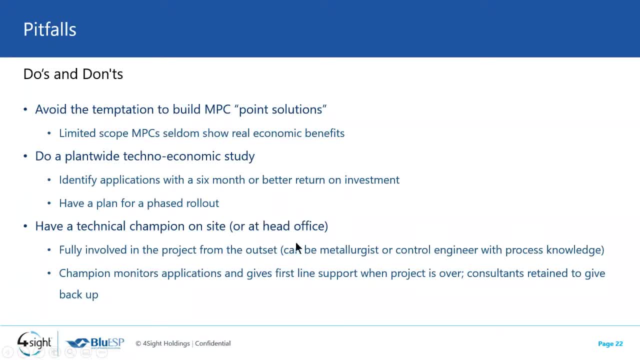 Have decentralized staff- Okay, Thank you very much- site or nowadays, as we've learned i think in the last months or so, we can work remotely with the right connectivity, but have someone from your company, your operation, fully involved: can be a metallurgist, a control engineer. this person monitors the applications and gives first-line. 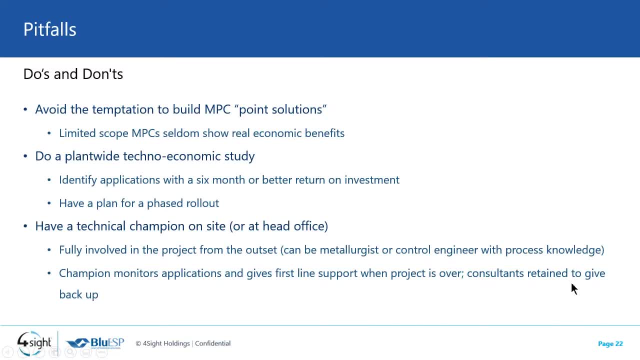 support when project is all over. you may want to keep the consultants to give some backup, but this is a very important role. shouldn't be a part-time role of of a dcs engineer somewhere that doesn't work well. change management is very important in these projects, as in. 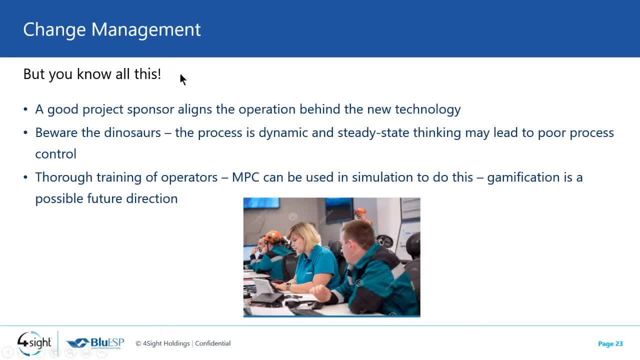 most software projects. so i'm sure you know this. but have a good project sponsor that aligns the operation behind the new technology. beware of my colleagues who think steady state only. the process is dynamic. that's why you need a control system, and the more dynamic it is, the better the control system you need. 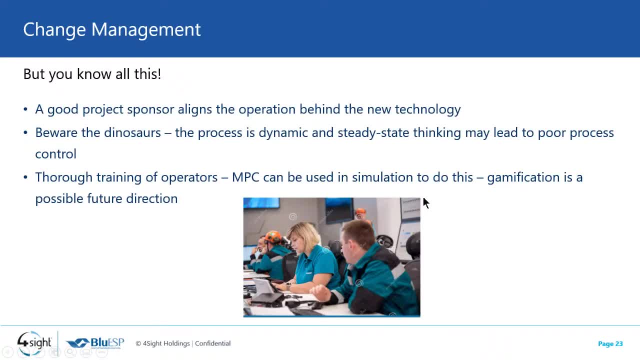 and do thorough training of the operators. npc is great because it is a model of the process. inherently, you've got a simulator, so you can use the simulator for training and in the future i'm sure that gamification will be used to improve these, these trainings, and to 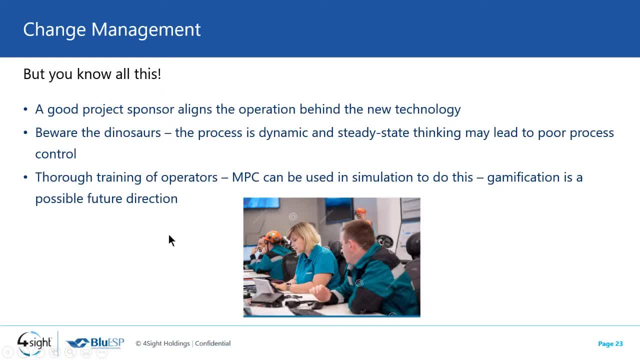 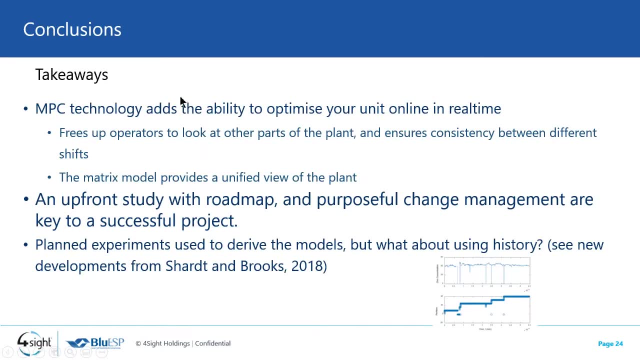 make sure the operators make the best use of the tools. so, in conclusion, npc technology gives you this opportunity to optimize in real time, minute by minute. we run the things, in some cases even faster than once a minute, and this matrix model, that picture i've shown you, gives you a unified view of the plant. 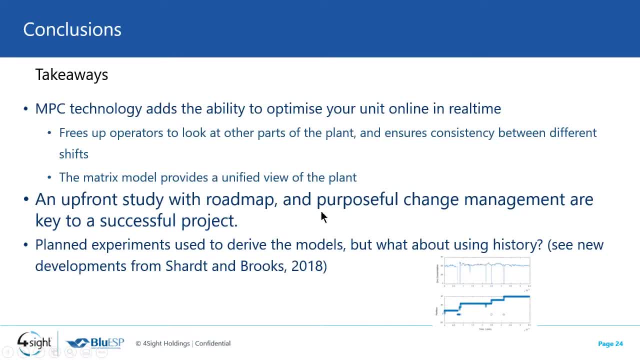 that you can use for other studies. an upfront study with a roadmap and purposeful change management will get you there. um, we've talked about uh. villalum talked a little bit about ai. i haven't talked about it because i've been looking back rather than forward, but my one: forward look. 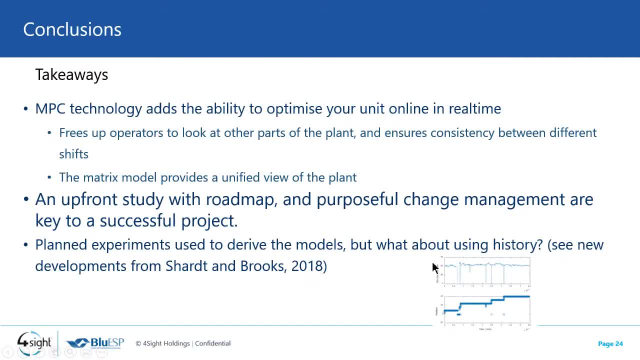 is about the large amount of history that you people already have it from your plant in your historian. and why aren't we using that to develop models? and there are good reasons. it's difficult. it's hard to trawl through manually, but i am doing some work with a colleague in 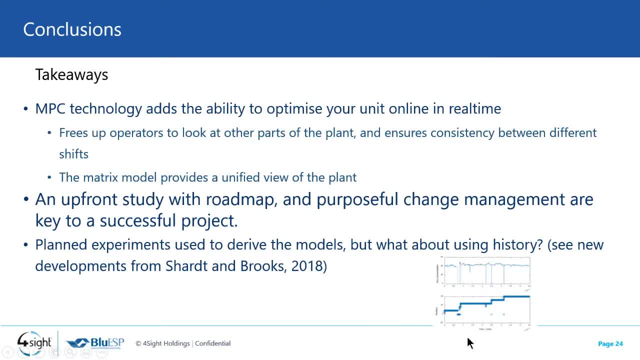 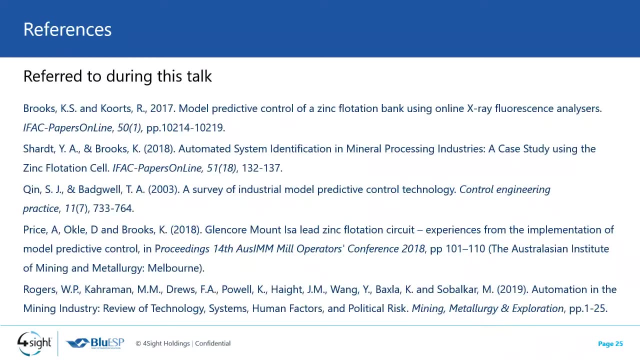 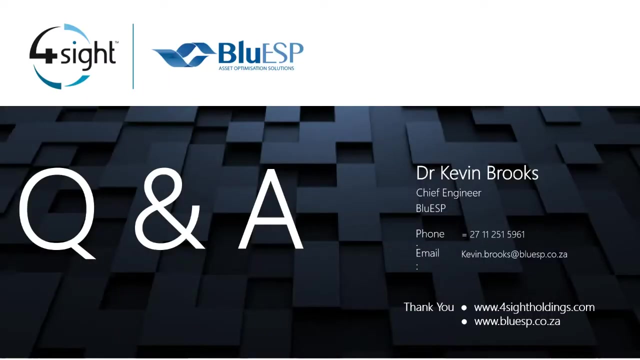 germany, and we've published a couple of papers. this is the first one where we use sophisticated techniques to slice the data in a way that we can then use it for model identification. so thank you very much. there are the references that i've used during this paper and, without further ado, i'd like to move into the questions and answers. so back to 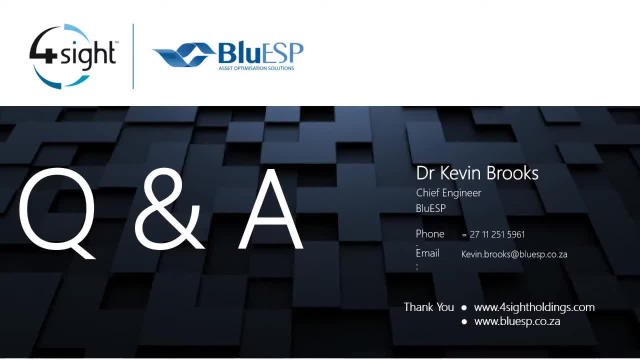 mirinda. thank you, kevin. thank you for that very insightful presentation. um, i'm sure everybody's found it extremely useful. um, i've got a question here from somebody who's asking: uh, what would i do if my process is really very non-linear? yeah, and what we found is that there aren't too many very non-linear processes. um, 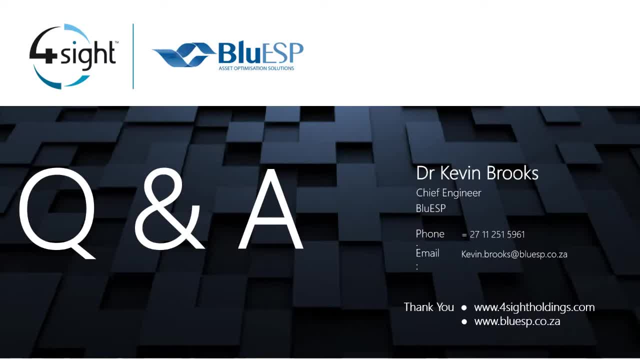 so the, the linear technology, has feedback in it. so we develop these models and and while we're running, we are adapting them as we run, by putting feedback into them, and provided you do your step testing around the area where you normally run, um you, the, the linear models, manage fine if you have. 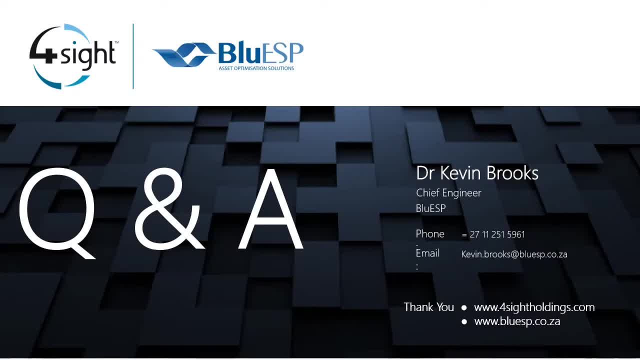 a real non-linearity and you know what it is. you can build it into the, the models, in a number of ways. you can use game scheduling or you can build a fully non-linear controller. but i would say, in a number of ways you can use game scheduling or you can build a fully non-linear controller. 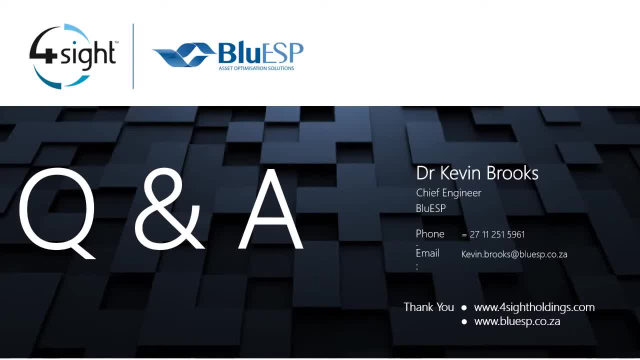 without thinking about the benefits of the non-linear controller, and you need to use game scheduling to make sure that that kind of dynamic communication is really easy to get across in your process. and, uh, we were also asked about the benefit of the non-linear controller for many of the products that we've been working on, um and we've been asking about. is there any? 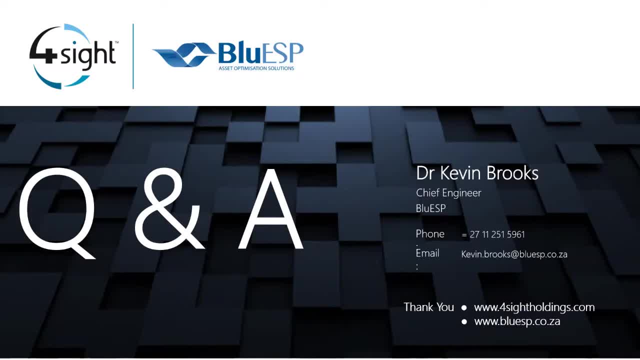 benefit of the non-linear controller, and i think the answer to that is no, but i think it's less than five percent of applications need that. another way of looking at it is is the 80-20 principle tells. We've got another question here. You talk about doing studies on the plants. Do you ever recommend that X-ray instrumentation should be installed for the MPC? 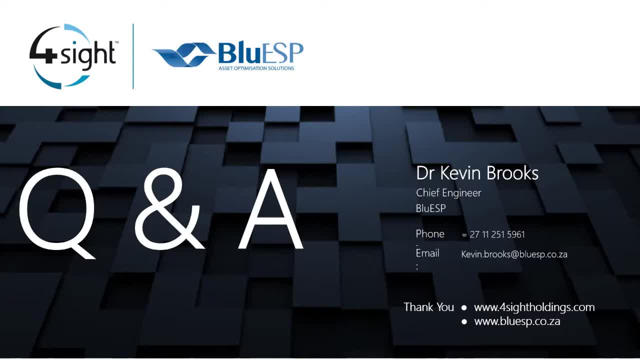 Yes, I mean that does happen, That during the course of the study we say: well, we can do some stuff with the instruments you've got, because almost always you can. after all, the plant's being run with that stuff. 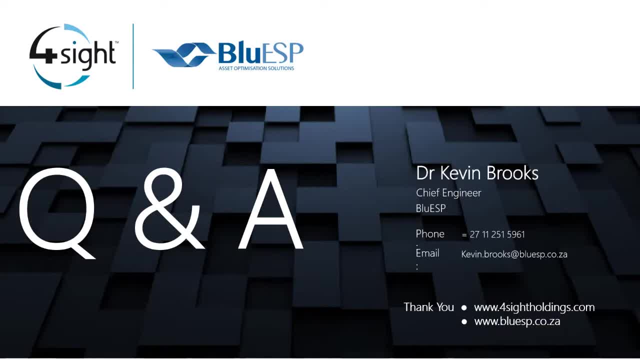 But that if you put this instrument in, then you will do a lot better. One example that comes to mind- Maybe a trivial example, but one that makes a big difference- is oxygen in the flue gas from a boiler. If you can measure that, you can really do optimisation of the boiler. 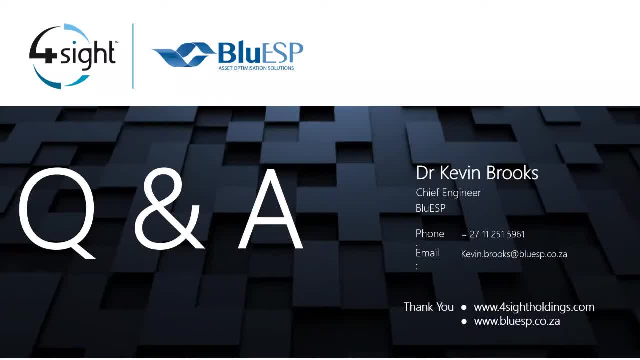 So yes, we do do that, OK. And then there's another question that's related to instrumentation. If you have a laboratory value that you only measure Once every hour, could you use that in a MPC system? Yes, you can. 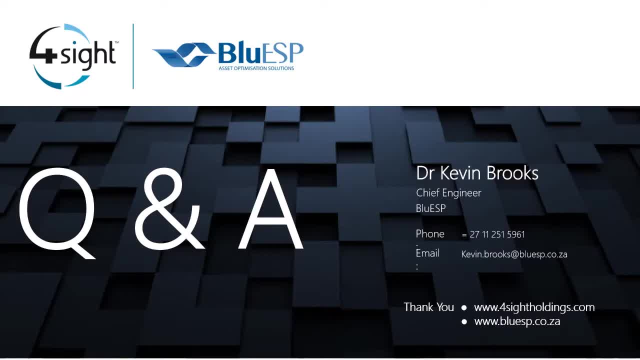 This is the field of inferentials, or soft sensors, that I've not talked about at all here. Maybe I should have, because it's been a big part of the gains that we had in the system. So, effectively, what you do then is, if you say you've got a lab value that's measured every couple of hours, 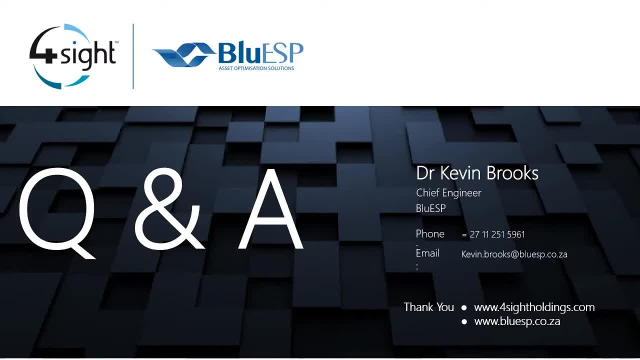 We use these new powerful statistical techniques- Supervised or unsupervised learning- to develop a model that's based on the process inputs that we do have- temperatures, pressures, flows- And then, when we get the lab value, we use it to update the model. 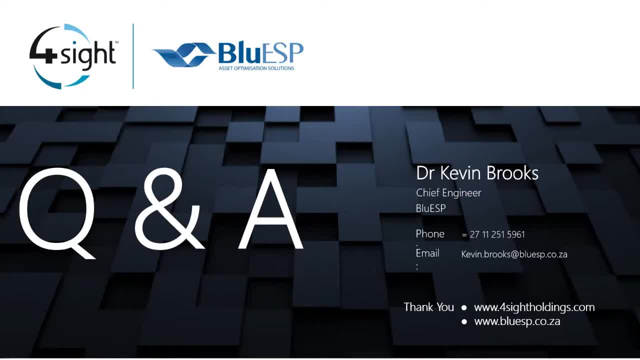 So it's a model controlling a model, and that works very, very well. It's been very effective all over the place And as the Um A I M Machine learning techniques improve and are easier to use and more robust, the soft sensors are going to become more and more important. 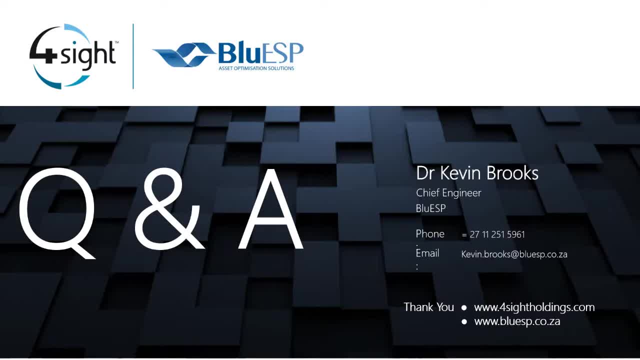 Yes, absolutely. Um, especially in the mining industry, instrumentation is a is an issue. There's a question here from Robbie. Can you comment on instrumentation in mining? Is this a limiting factor for MPC in general? Uh Yeah, it's hard to answer a general question, but yes, I think there there are things. if you come from the oil refining world and and then you, you, you find yourself doing this kind of work, it is noticeable not necessarily that the instruments are not as good, but the instruments don't work all the time. 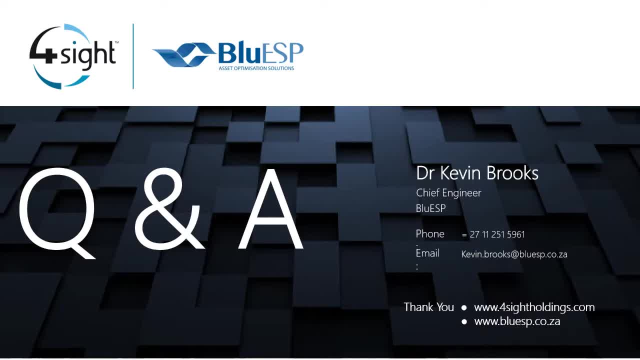 So, So that's something you've got to take into account that I think, because of harsh environments and and slurry flows and so on, like that, then the instrumentation does become an issue, and then it is an issue with, with online analysis. I think where we've had our great successes has been where the online analysis has been good, robust, robust, robust, robust. 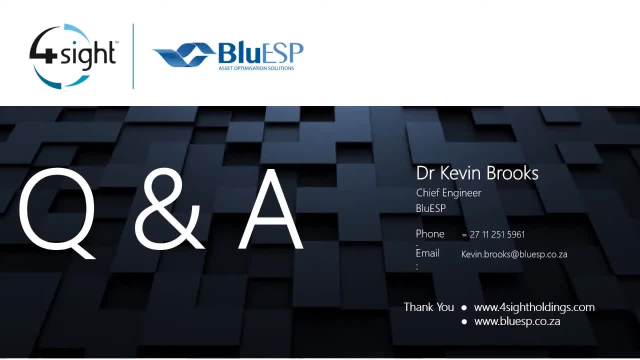 The instruments have been properly maintained and calibrated. Yes, Okay, I think there's one more question here, a very interesting one, Kevin. Um, how does MPC fare in processes that involve constraints that cannot be measured live, for example, a process involving biological constraints which take a few days to measure? 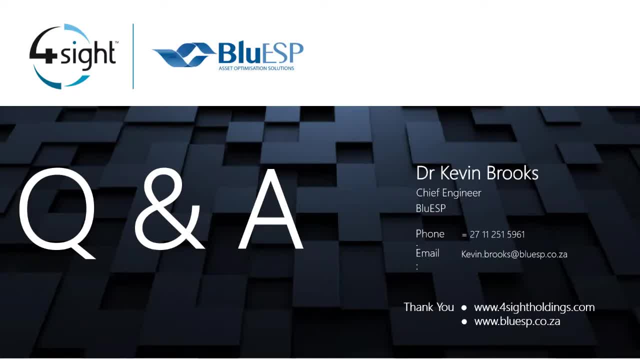 Yeah, those are very tough. Yes, So again you've, you've got to appeal to the, to the inferential world, And then what you say is: I'm going to do the best inferential I can, Right, And then I'm going to control conservatively because, if I know, I'm only getting an update on my measurement in two days. I'm going to have to stay away from the constraints by a fair amount in order to allow effectively for what is the noise in my measurement? 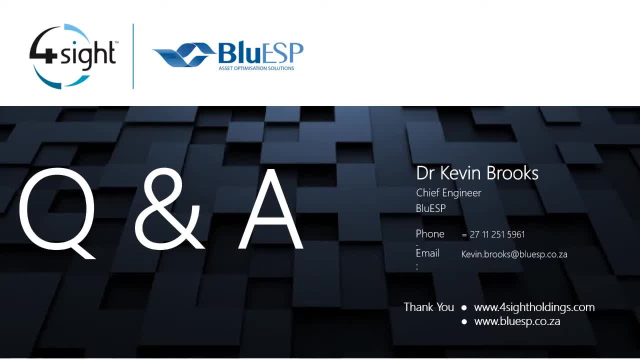 The error in my measurements, And that's a very tough one. I've certainly done, certainly done, applications where the measurements were shiftly, which largely means once every 12 hours. But even then you've got to be careful that that your inferentials are accurate and and that the updates are done. 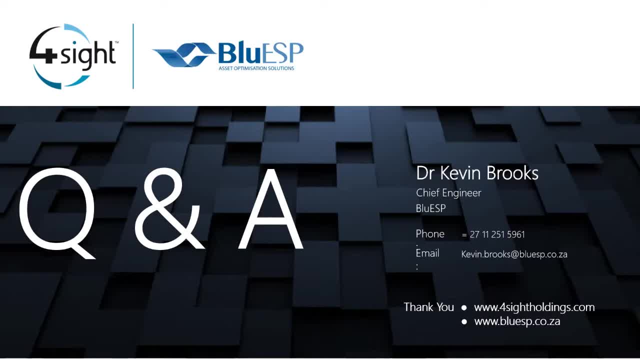 You might In that case want to suggest to the plant that that the lab frequency be increased to twice a shift, because that would give you a better comfort zone. Yes, Yes, And then we've got a question here. Do we typically write extensive logic to account for edge cases that might occur? 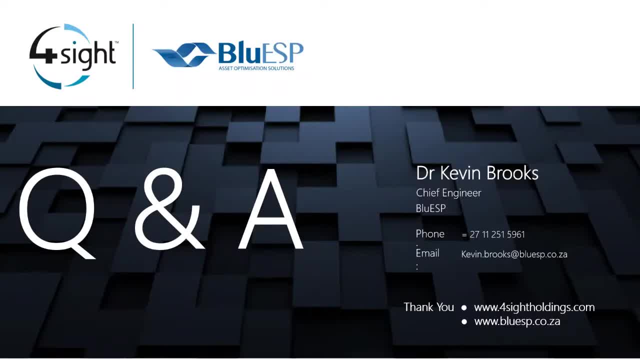 So how do you decide that the control is too uncertain and should probably avoid. So how do you decide that the control is too uncertain and should probably avoid Taking any action at all? fall back to the base layer, Okay. Well, I kind of hate doing that. 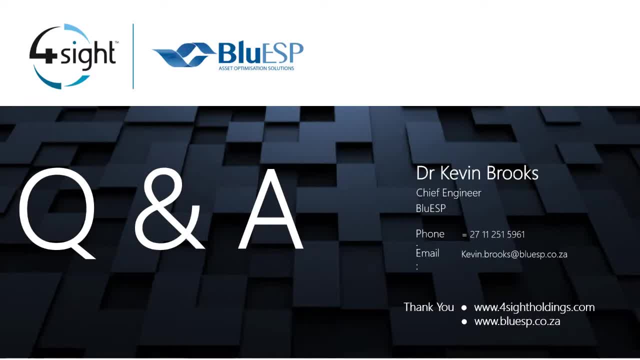 So, yeah, I'm not sure, Yeah, but it can happen. and and there's, there's always two levels of those sort of things. One is the automated level where you say I'm if, if this And this happens, I'm going to effectively say I'm out of here and, and remember, these systems cascade onto existing base levels. 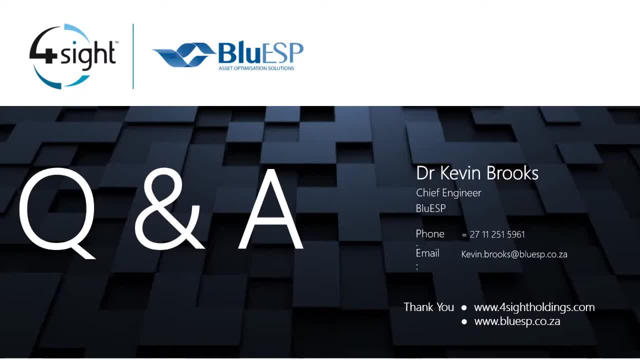 So there really shouldn't, there shouldn't- be a safety issue. switching them off, You lose optimization, You don't do safety. So it might be that you have interlocks and things like that that will switch the system off, or something I prefer actually is. 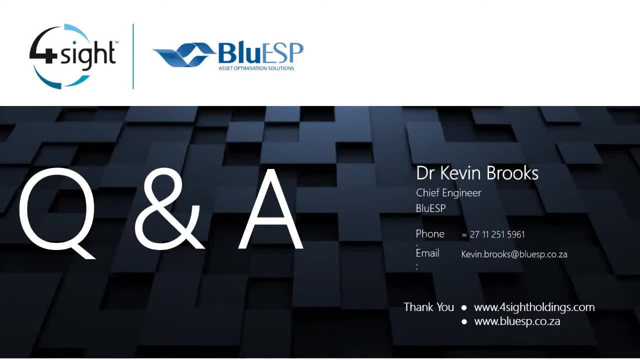 To count on the operators. The more you count on operators, the better job they do. So if you say to them: look, I'm giving you this thing, and generally the operators like the NPCs, But you need to watch this and this and this, and if this happens you can take control, 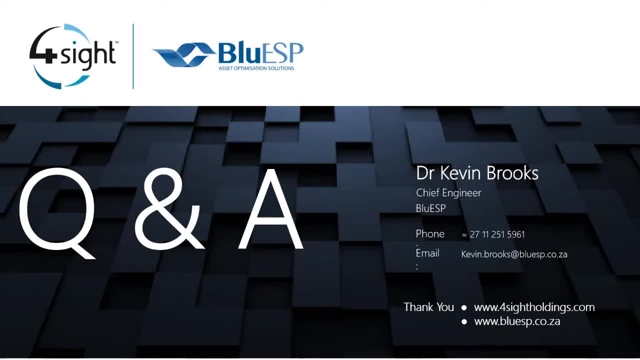 Then I think you are treating the people who who are running your multi-billion Rand plant as adults and and giving them responsibilities, And I think That generally works Well. you can be very sophisticated with interlocks. You can do lots of clever stuff, but 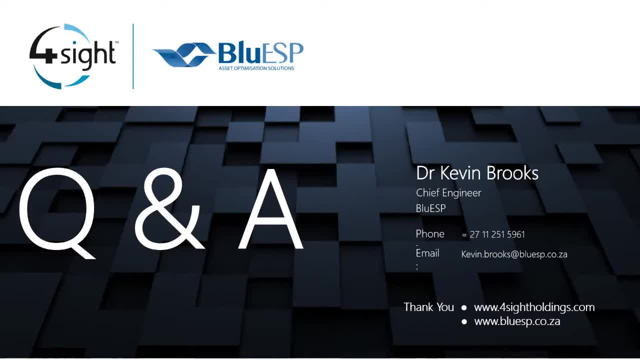 There's a cost element to that. Yes, Yeah, I think the measurement seems to be quite the topic. here Is another question about how you handle. is it possible to safely handle instrument failures with NPC controllers? Do these have to be built into the controller initially? 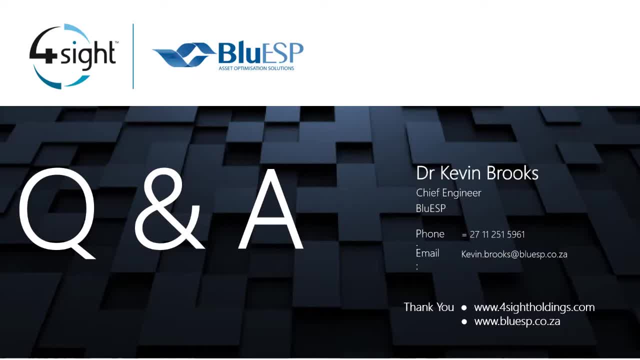 So another field I'm extraordinarily interested in- and I've published a paper with Professor Bauer, who was at the University of Pretoria, where we looked at sensor validation, and we did this even before the Boeing 737 Max issue, which was effectively exactly that issue- 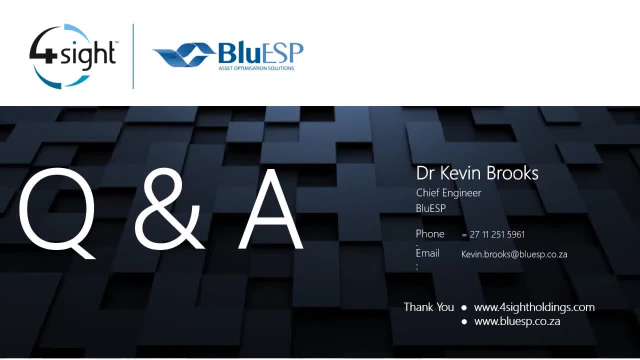 And, yes, you have to Validate the instruments That could cause you issues And and it's very tricky because it inevitably involves setting up limits and rates of change and and that's not a, that's not, in my opinion, not currently a great science in how to do it. 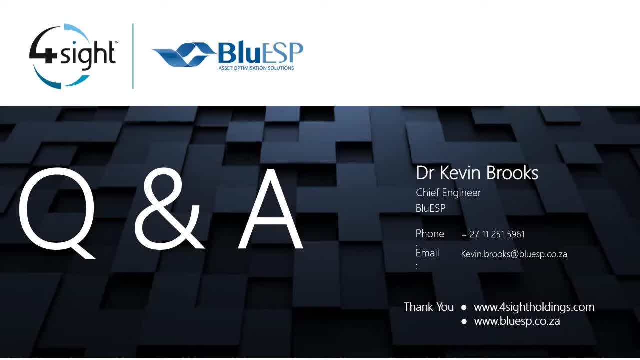 But yes, you do have to do it, particularly with the, with Analyzers and so on, which which you know can, can drift and and give problems. Yes, I think we have time for more questions. Here's an interesting one. 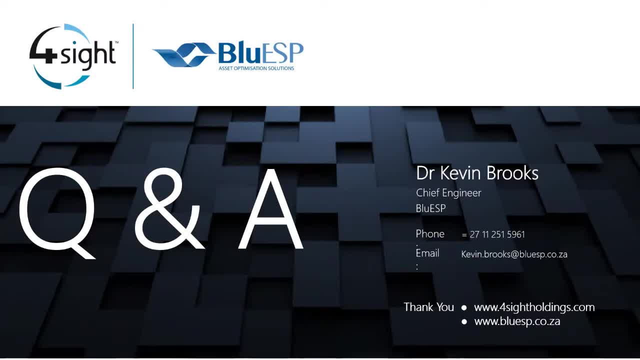 Kevin, in your experience, if you had equal success implementing NPC technology with rigorous models as much as you have with empirical models, even that plant engineers tend to be difficult fiddling with their processes, live I've, you know I, in 25 years of doing this, I've, I've, I've not done one project where where all the models were rigorous. 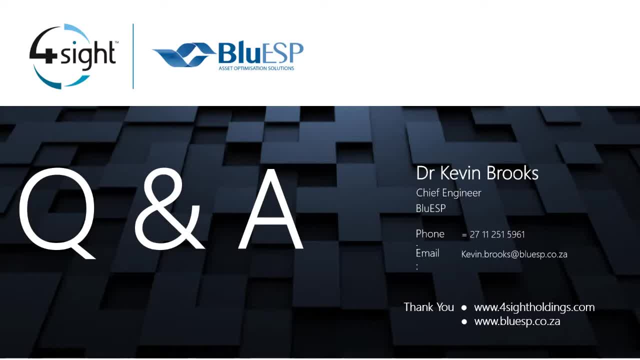 So where we might use rigorous models is where it's a fairly simple calculation. level in a tank is a good example. So if you know the flow out, if you know how the change- there's a change in the flow out of a tank- and you know the size of the tank and where the level tappings are, 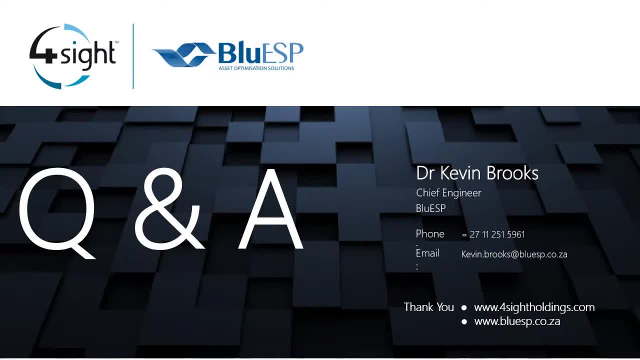 You can calculate The change in level. density is another one where you can often do the calculation. But apart from that, we really have found that the empirical approach is better. We we trust our models, We can interrogate them, Everybody can review them, and 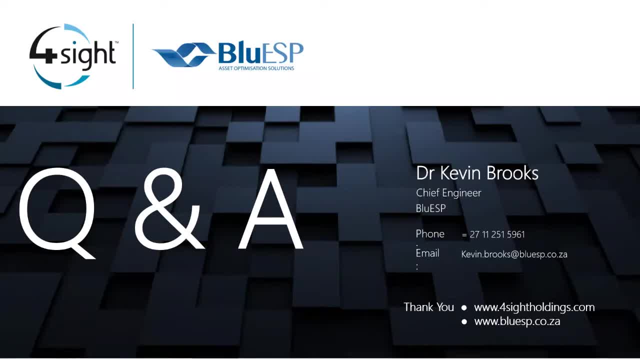 And and they're developed in a in a time span that is reasonable for these projects I mean. otherwise you're looking at masters and PhD level stuff to develop a model and that takes The best masters you're going to get done is in a year. 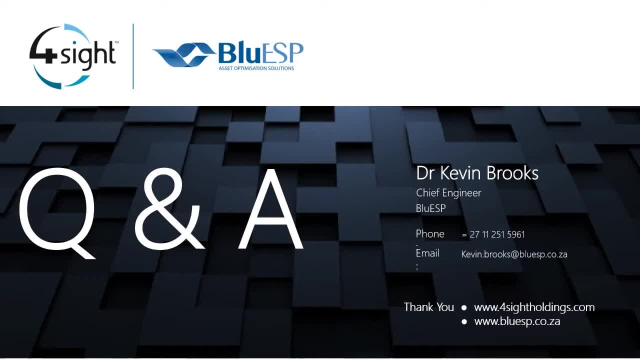 We don't have a year to do the project, So I'm maybe overstressing the case. There has been some work done in very big distillation columns where step testing is difficult. So if you are interested in this field, you can. you can look for some work by a guy called Jose Ferrer. 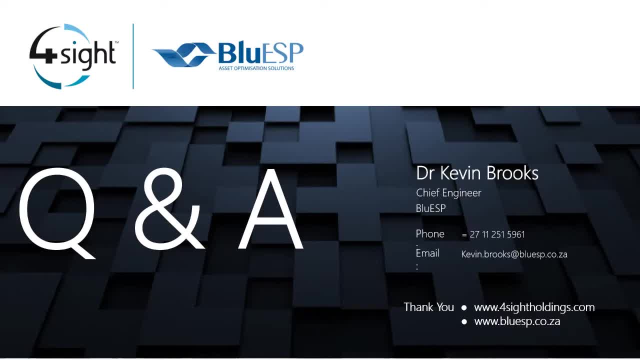 but that's very specialized, I would say Okay. and then a question here about noisy measurements: Does MPC work on processes with noisy measurements? Yes, fortunately it does. I don't know if you remember there was one little picture I put up where, where the trend looked sort of 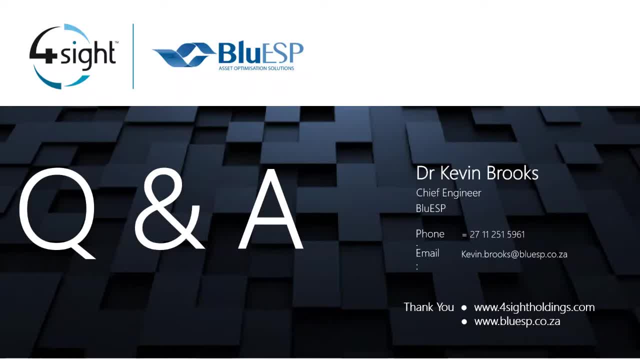 was moving around. There was a blue trend and a red trend. that would be because of noise. But the way we do, we derive the models using these FIRs. FIR is a filter, So we we do get get rid, We do derive models despite noise. 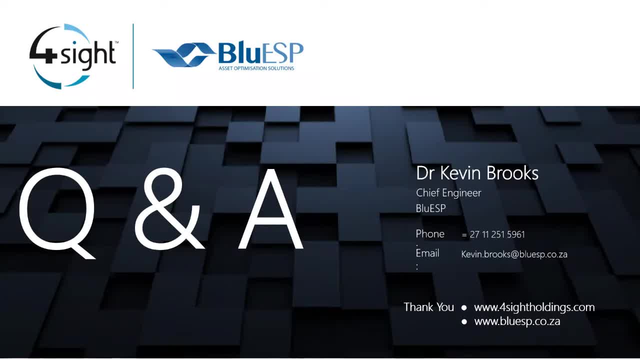 Obviously, the more noise, the more testing you need to get the models. If the signal is too noisy, then then you have a problem and you may need to go back to the signal And maybe do some filtering on on the signal in the DCS. 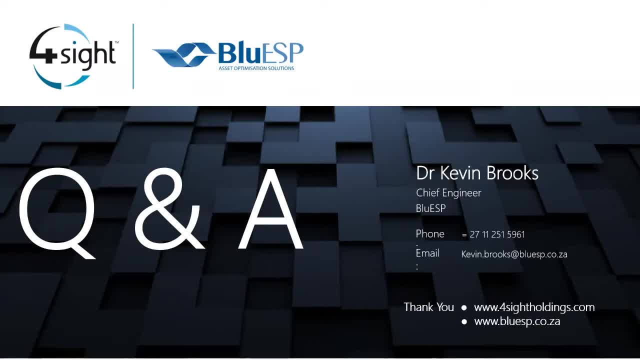 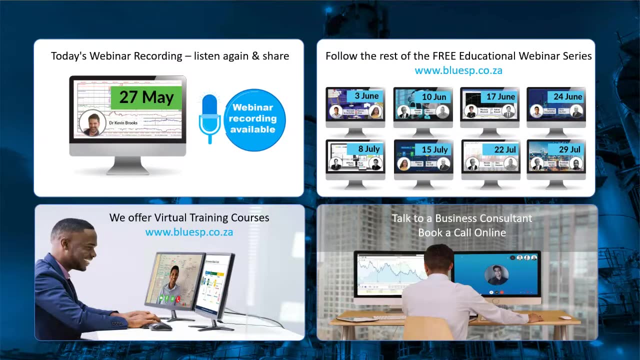 Okay, I think we have time for one last question. Yeah, When questioning a control room operator, why turn the controller off? The common response usually is: I didn't know or trust what the controller was doing. Have any? Do you have have any? easy to understand? 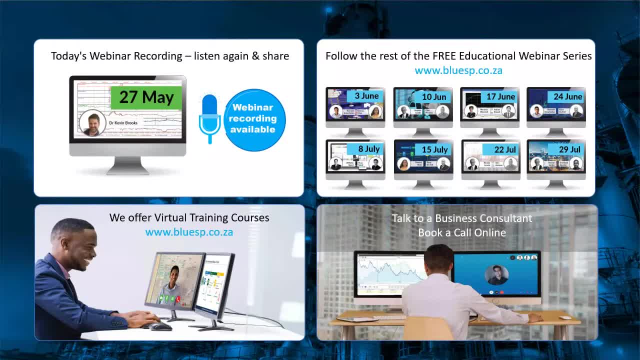 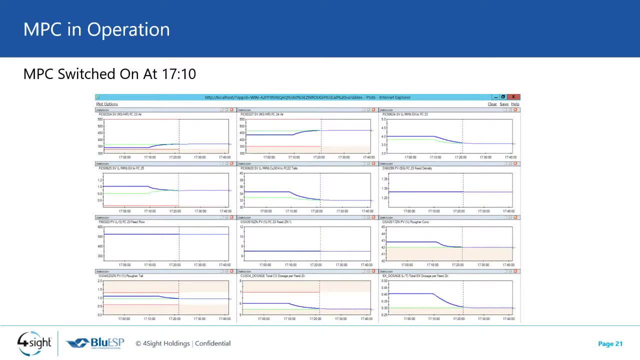 Visuals been worked into skater pages to reassure operators of the action the controller is going to take. Okay, that's a great question. I'm going to just go back to one picture here, if you don't mind, because that picture That is a simulation and and we have colleagues who are very clear about how careful you must be about simulations- 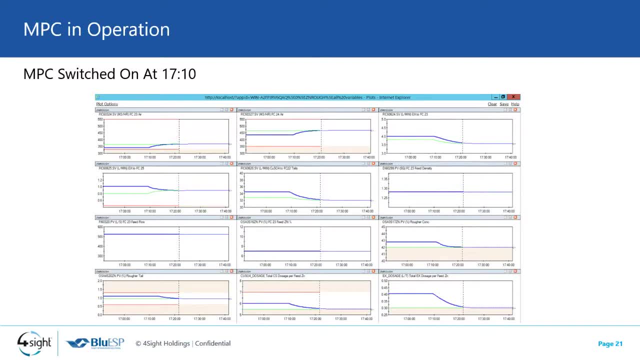 but that picture is on a television wall on the control room in Mount Isa Because it shows what's going to happen in the future, At least what we think is going to happen in the future, And that, in my mind, trends like that- Oh what it? what is key for a human to understand what's happening with the process. 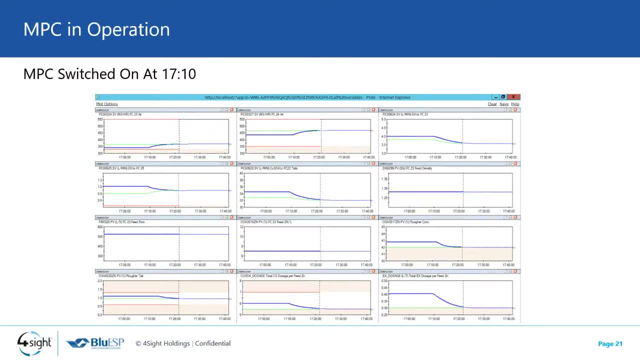 So this trend can be formatted how you want. You don't have to put in all the all The plots, and you probably don't want it bigger. I think we can do six by four or something on one page. The 24 plots are plenty. 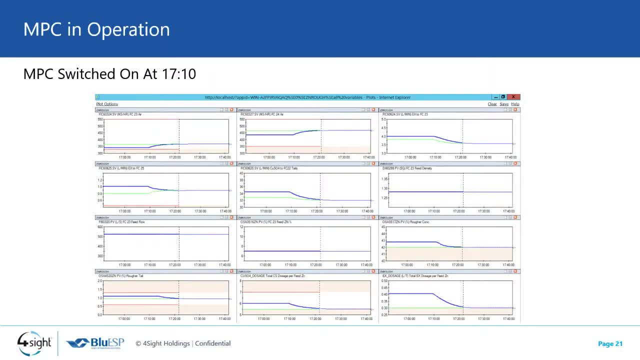 So, yes, I think there are tools And, if used by sensible operators, I think they lead to interesting discussions as well when you're commissioning Of of, because- because the operator can see what the system is Doing It's it's quite transparent. 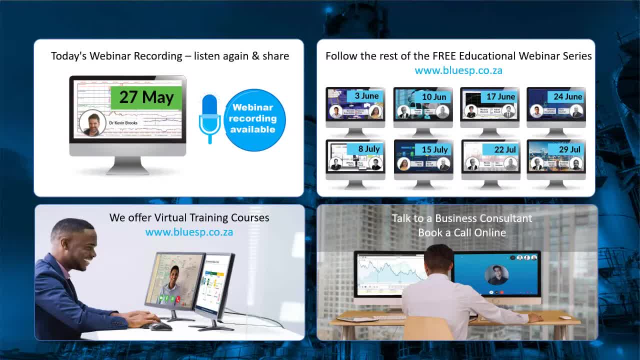 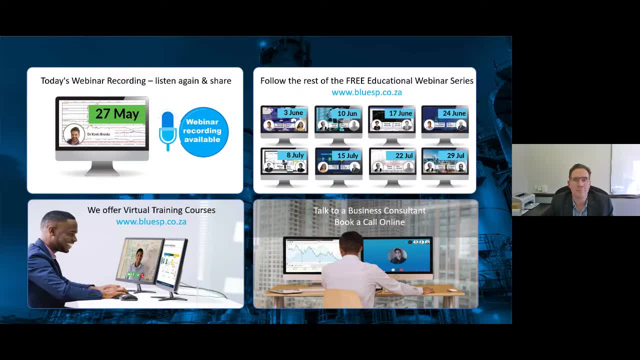 Yes, Thank you, Kevin. I think we've run out of time for questions. Thank you so much for for your very insightful presentation. If anybody, if you have any more questions or anything you'd like to ask Kevin, you're welcome to send him an email or contact any of us, and we want you happy to answer any questions. 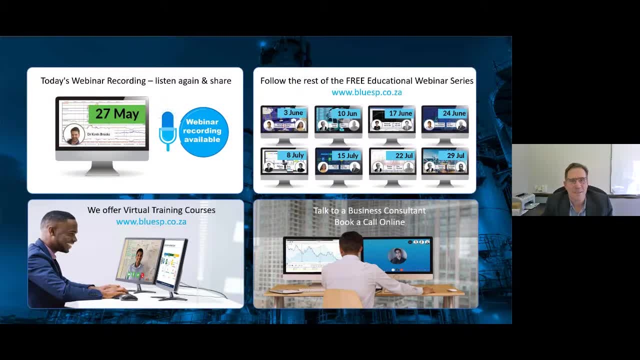 You have over to you. Valellum, I think you want to make some closing remarks. Thank you very much, Miranda. and Thanksgiving, What a great presentation. So thanks for the preparation and, and, you know, and sharing that information with us guys. If we haven't answered your questions yet, you can carry on typing and, Kevin, you know Miranda will get back to you in writing. 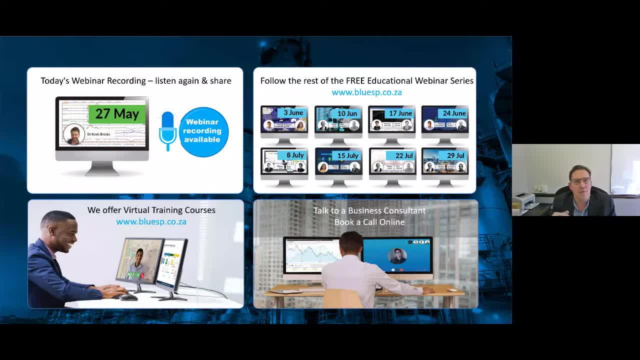 So this event is recorded, as you can see, and and so even if tonight you revisiting of you Share it with a colleague and he has some questions, that question will still come through to us because it really it lives on and you know, and and we will get the questions and we will get back to you with those answers. 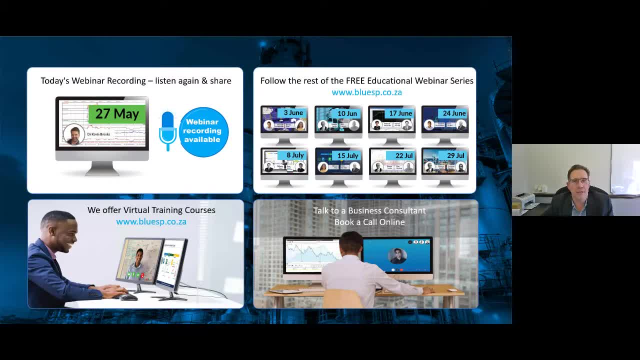 So please engage on, you know, on this event, or if you revisit it a week from now and you have another question, just type it in and it will get through to us and we will basically be able to answer you on that. So, and thanks for all the engagement. 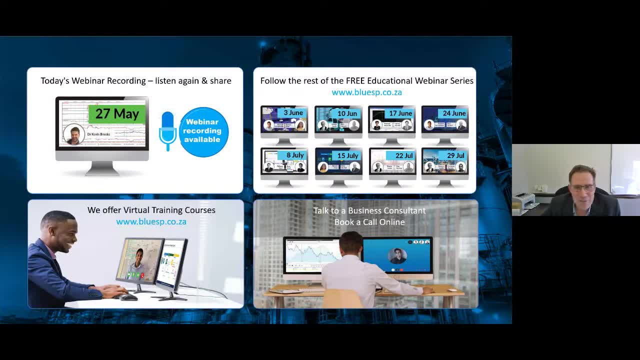 I think we were peeking somewhere Over the 90,. you know, I never knew there was so many people in there that so interested in in in Advanced Process Control. Maybe they just wanted to to hear Kevin. you know he was a lecturer in previous life. 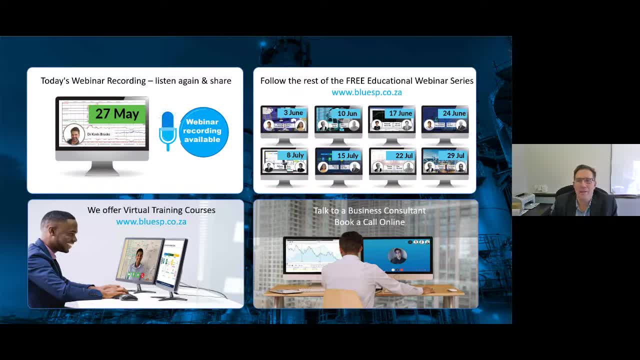 So a lot of his ex students probably want to also listen to him again. So that was, that was a great one. So I think the next theme is is there is many more of these events happening, So we're having another two Advanced Process Control events as well coming up. 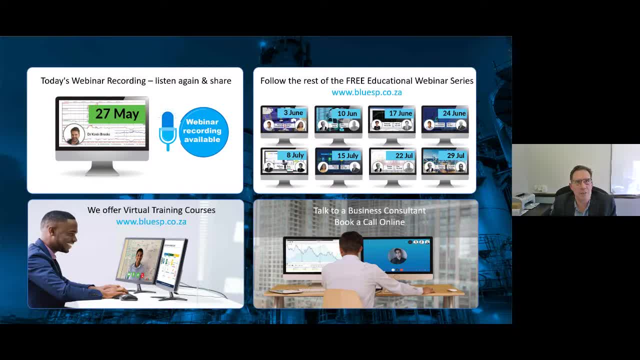 So so please follow the links again. So We'll send you a thank you notes after that. And there's more links so we can register for some of the others. So so we will at some stage still have Aspen. Tech presenters also talk about the vision, the future, the, you know, this combination of bringing Advanced Process Control into the tool of Advanced Process Control. 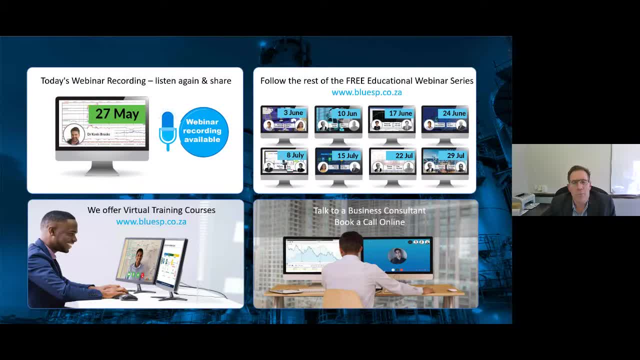 And so it would show you and share some of that technologies and we normally would do training on APC, DMC3 and that in our offices. obviously now with COVID 19, that's not possible but we carrying on with e-learning. So there is free e-learning to Aspen Tech clients up to the end of June might be extended again and also we doing virtual training. 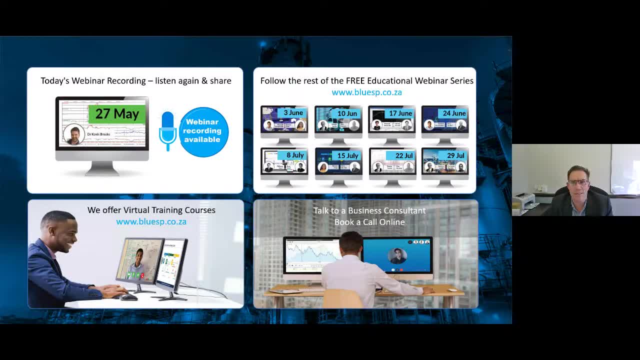 So last week we did virtual training for an audience, next week There is again. So so training carries on. It's just now in virtual space with a lead instructor. And then I think the last one is is if you believe that that anything that Kevin or Marinda shared with you is valuable and you would like